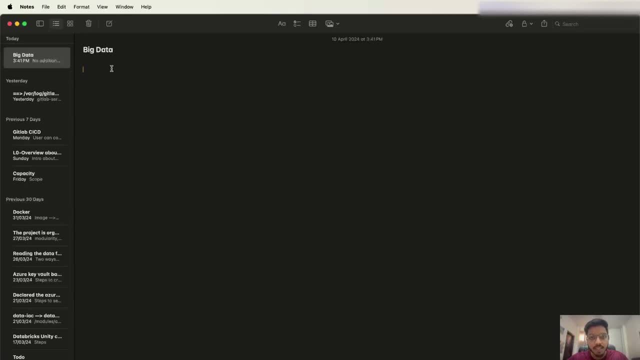 But what is that huge thing is like that is, is there any benchmark? or like is: when TB data is used, if 100 TB data is used, So what is that benchmark? So in the layman terms, we just say, okay, if the size of data is used, this is Big Data. 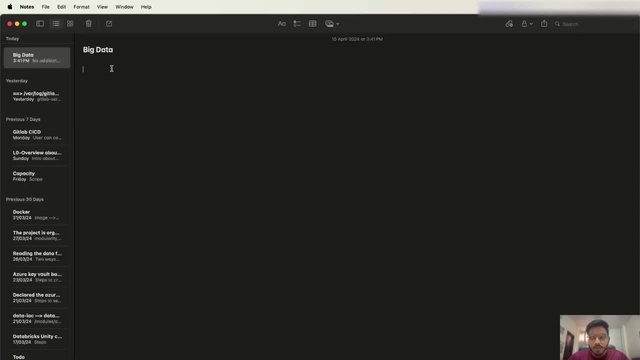 But what is that benchmark? We don't know. So we will be learning, like: how should we actually define Big Data? Is it directly, is just like? is the size is only thing that basically define the Big Data, or are there any other factors that contribute to this? 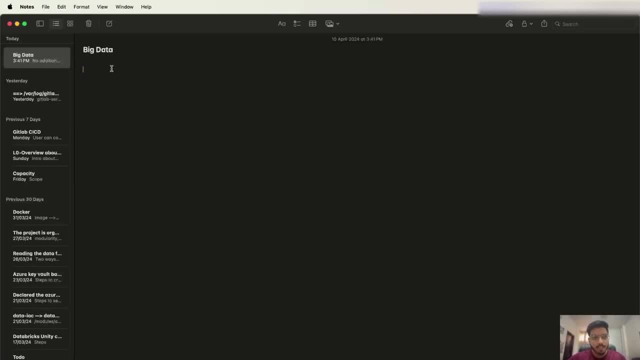 So we will be learning this And so if I tell you the formal definition, So the formal definition is basically: we have three V's to define the Big Data. Three V's definition is there and there is also five V's definition. 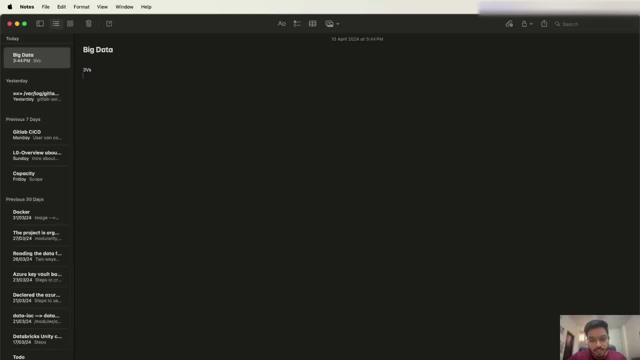 So I will like, I will focus more on the three V's. first three V's that are important. Other two V's you can explore by yourself. So these three V's are nothing but volume, velocity and variety. 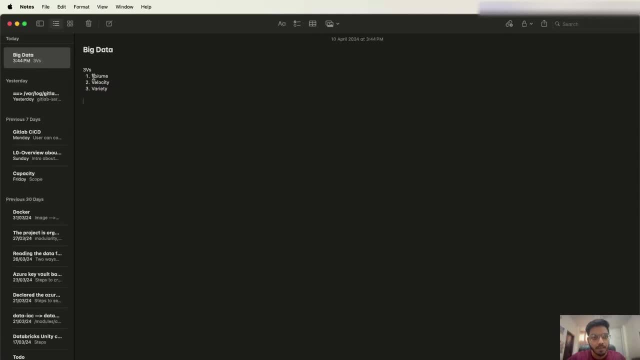 So these are three V's that we will be learning, So and these three V's basically define the if a data is huge, if a data is Big Data or not. So the first thing is volume. So suppose you have a system with some, let's say, 8 GB RAM, 16 GB cores, and let's say 1 TB hard disk. 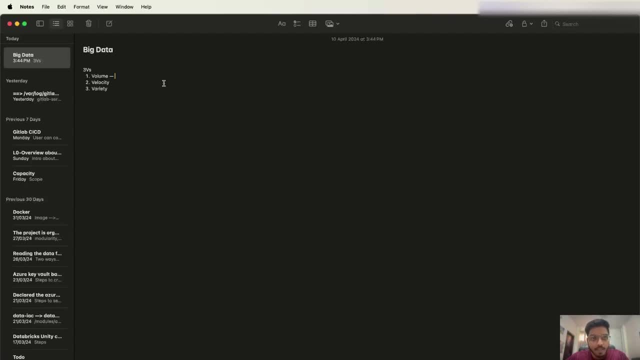 And if I give you, let's say, 100 MB data, MB data to process, you can easily process it because you have, let's say, 8 GB RAM. It will easily. it will easily, you know, fit in your RAM. 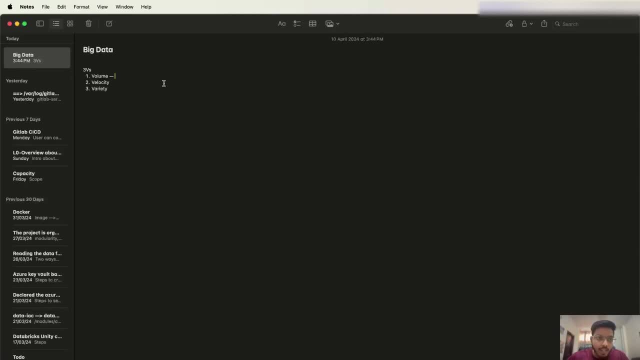 Because the data needs to be fit into the RAM. then only it will be, then only it can be processed. So, but what happens now? I start giving you, if I start giving you, let's say, 10 GB file and let's say 100 GB file, 1 TB file. 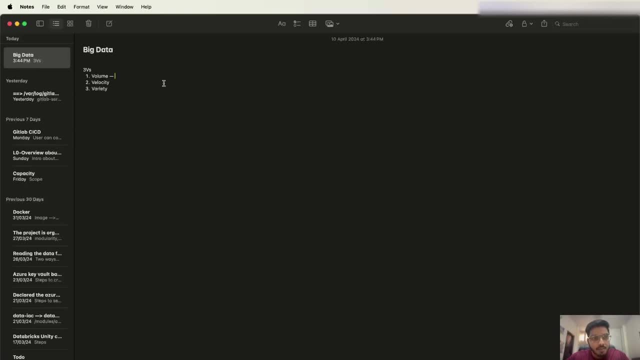 Now your system will suffer because the RAM and the processor thing is like very limited in your system And it cannot fit in your memory the size that I am giving you, let's say 100 GB. So your system will suffer. 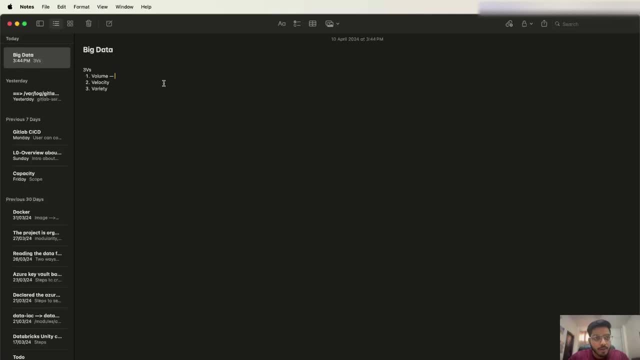 So if your system is not able to process a particular amount of data that is coming to you, then in that case we will say: this is our Big Data. So this is volume. Then now the second thing is velocity. 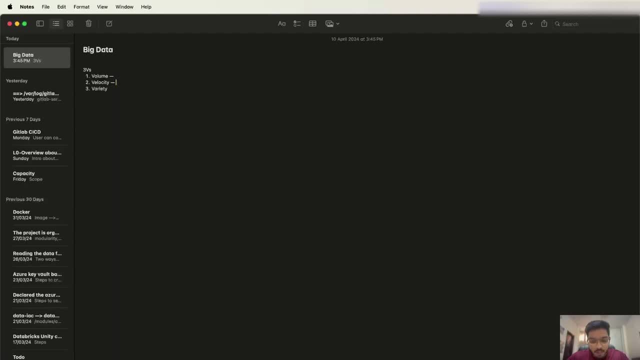 So what is velocity mean? Suppose, earlier I was giving you a single file only, let's say 100 GB file, But, and I'll just give you one file only. Now what I'll give you is, instead of giving you Big Data files, I give you, let's say, 10 MB file. 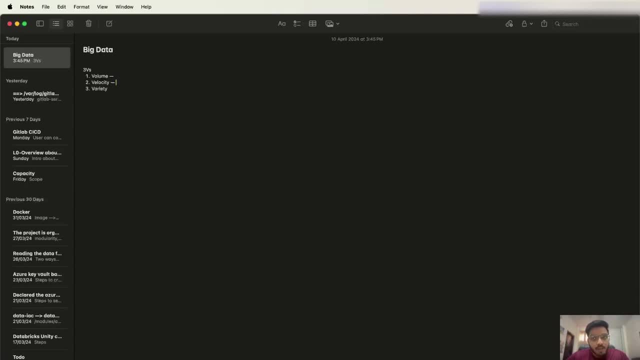 And I'll give you 10 MB file. on some regular interval, Let's say every 5 seconds, I'll give you 10 MB file And your system has to process the same. So every 5 seconds you have to process the same. 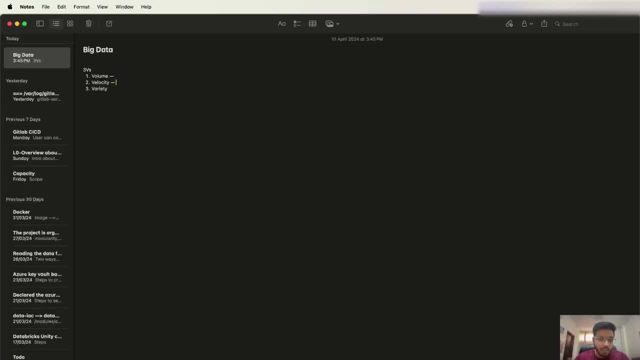 10 MB file, Because every 6 seconds you will be getting new 10 MB file And in those 5 seconds you have to process. you have only 5 seconds to process the 10 MB file And if your system is not able to process that 10 MB file in every 5 seconds, then we will say this is Big Data. 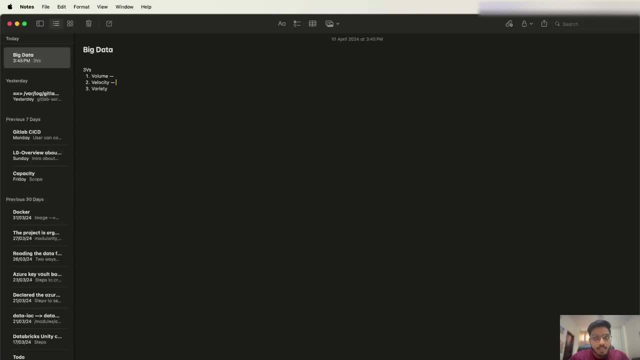 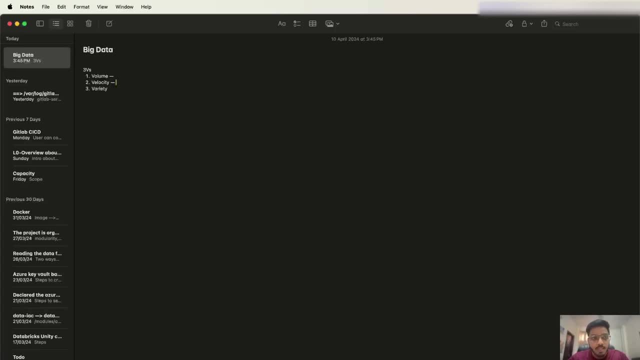 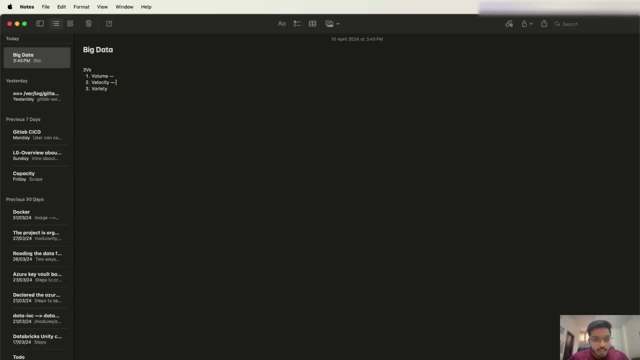 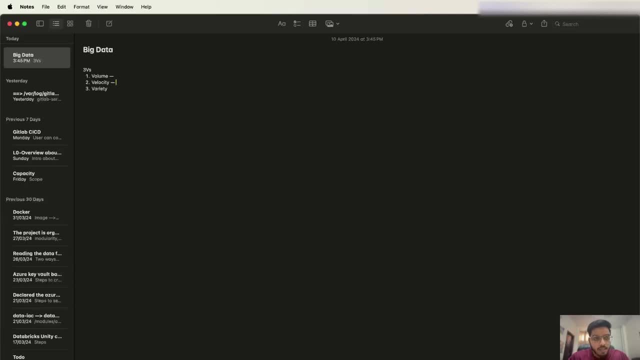 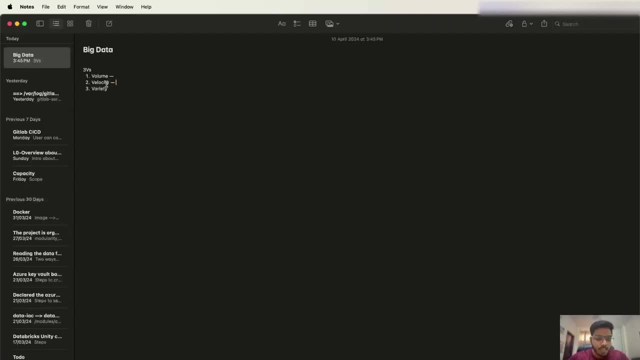 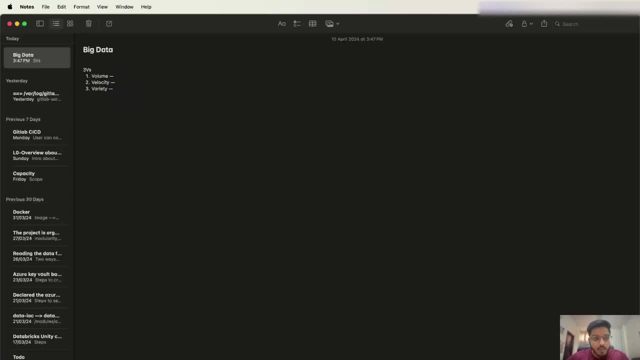 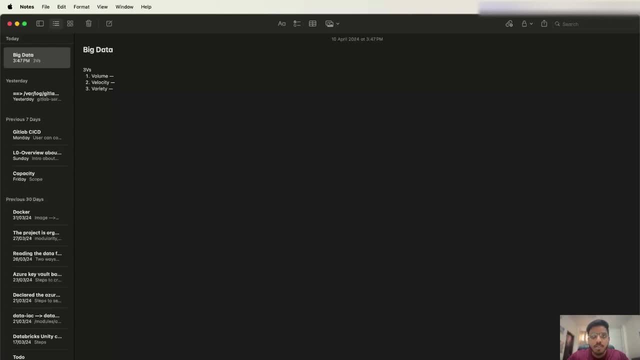 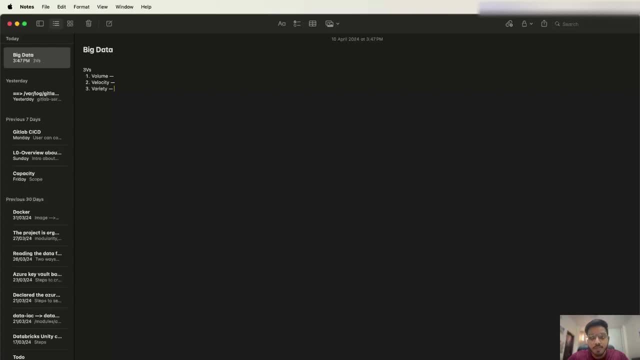 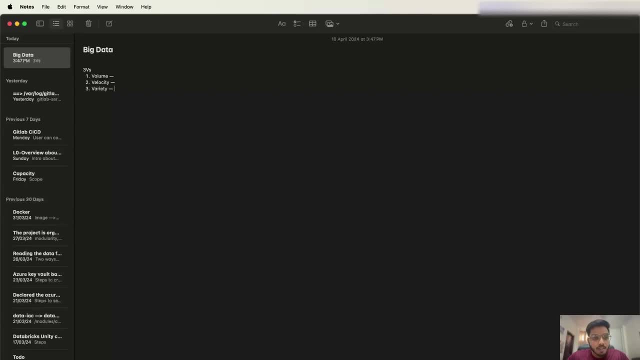 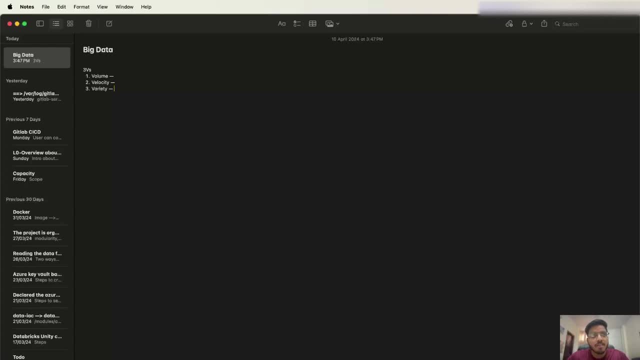 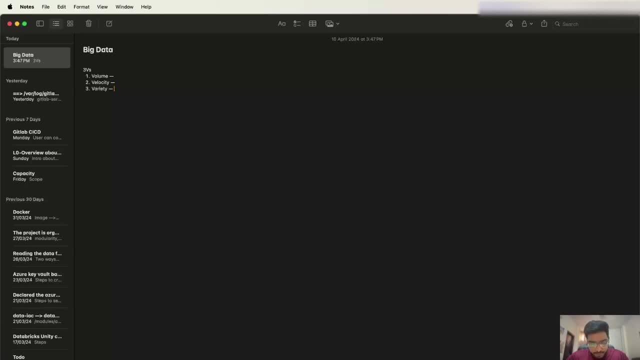 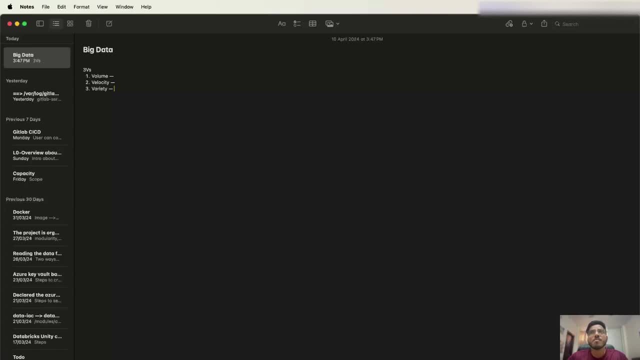 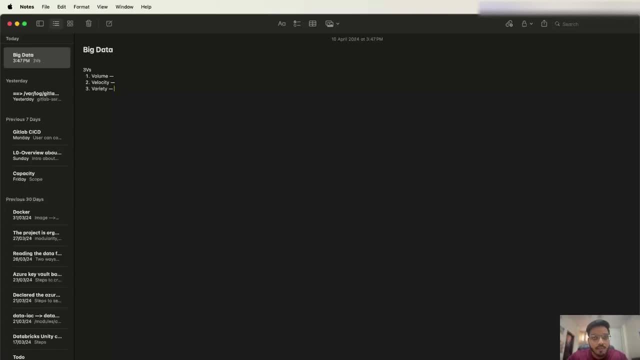 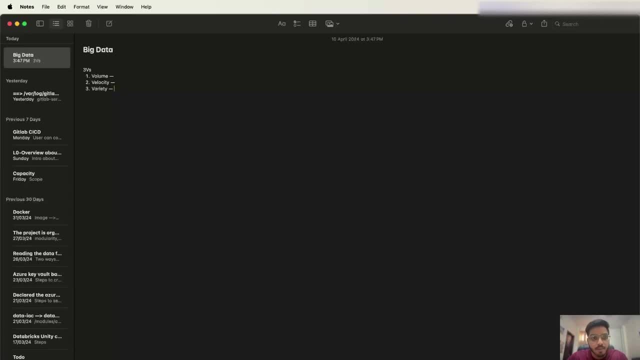 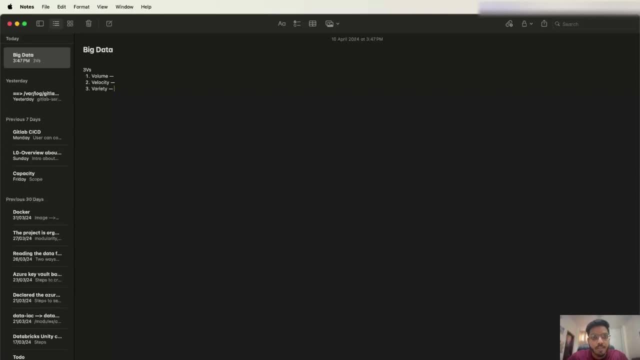 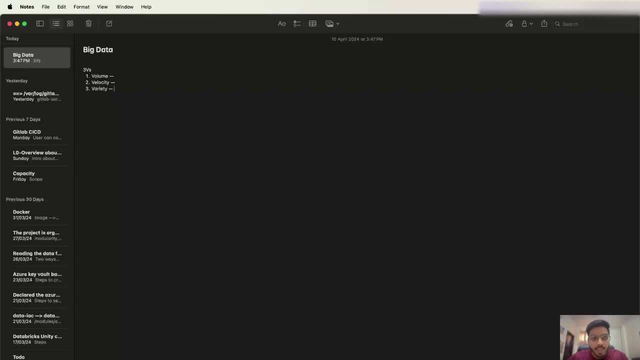 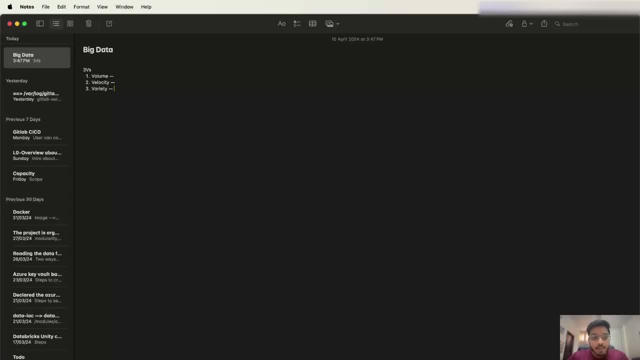 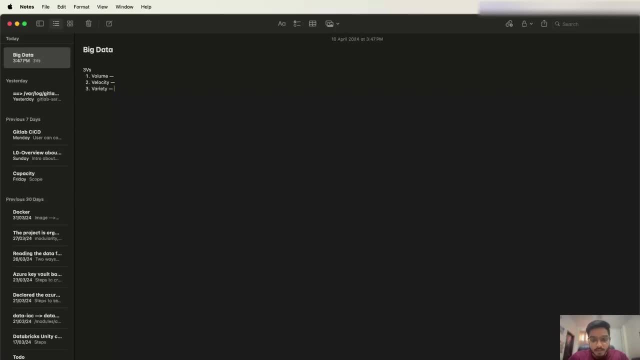 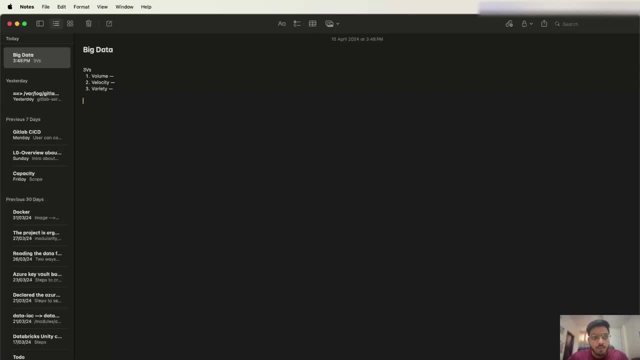 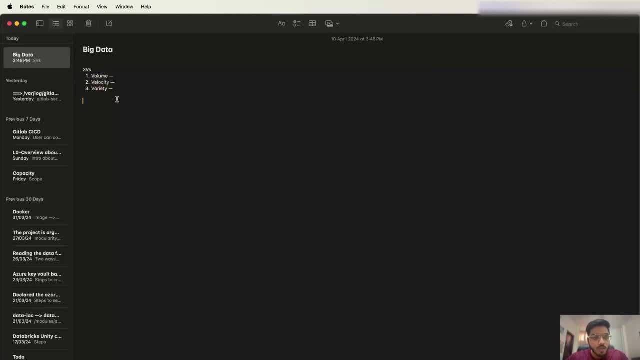 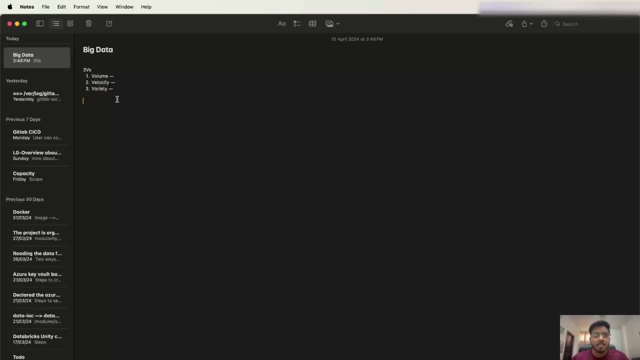 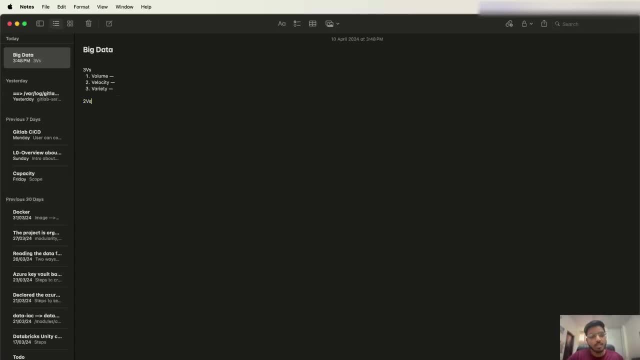 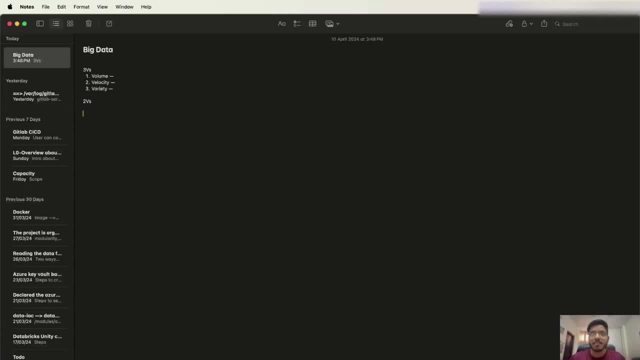 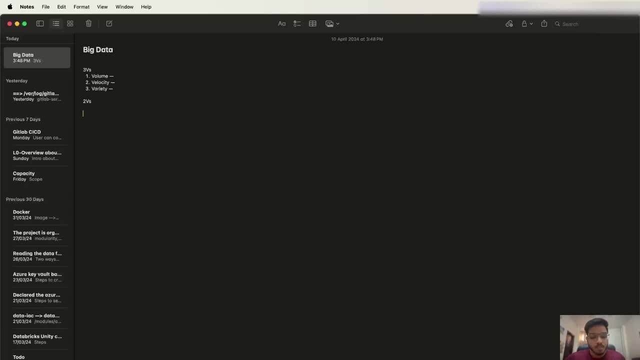 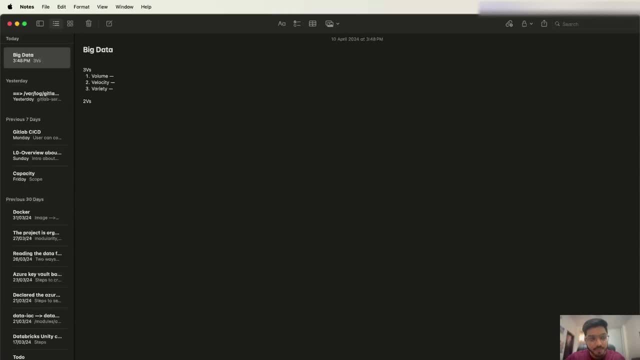 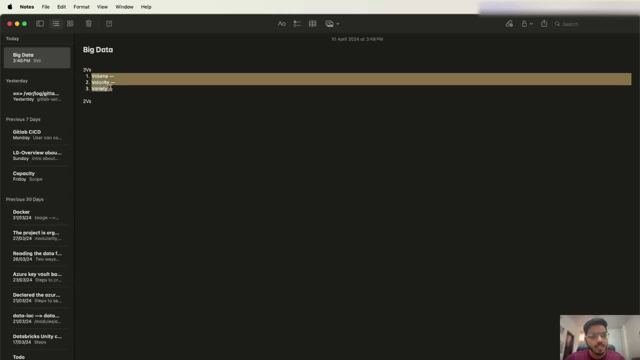 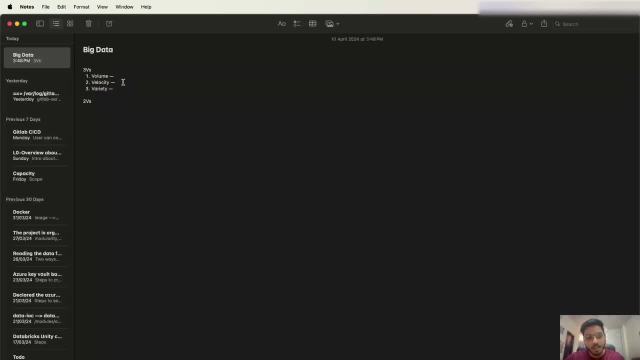 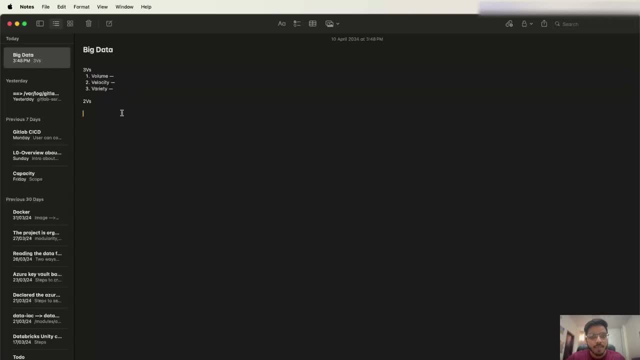 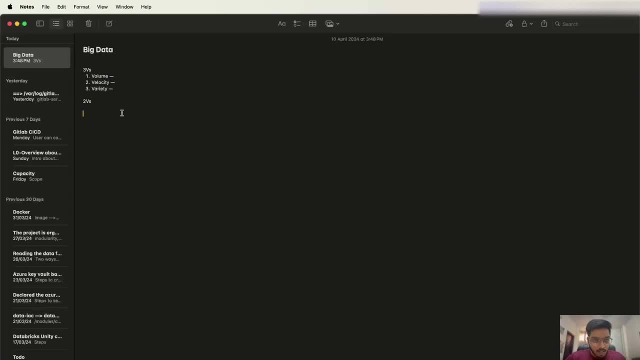 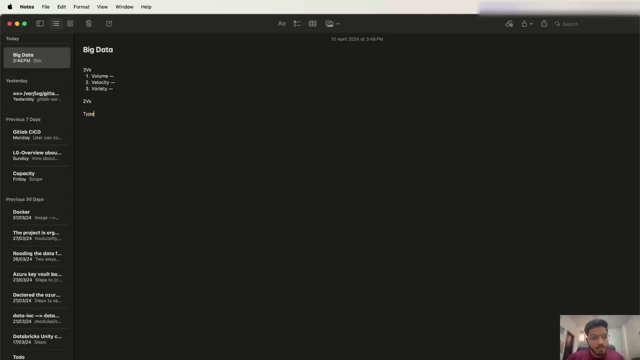 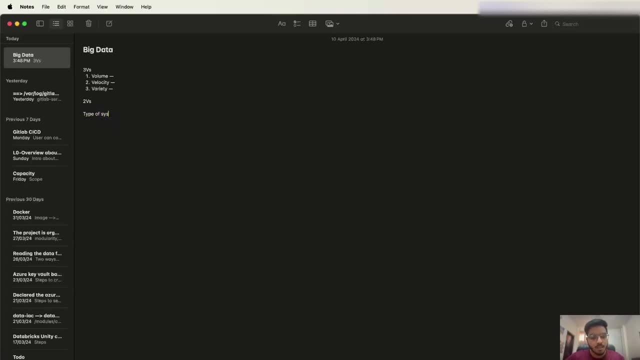 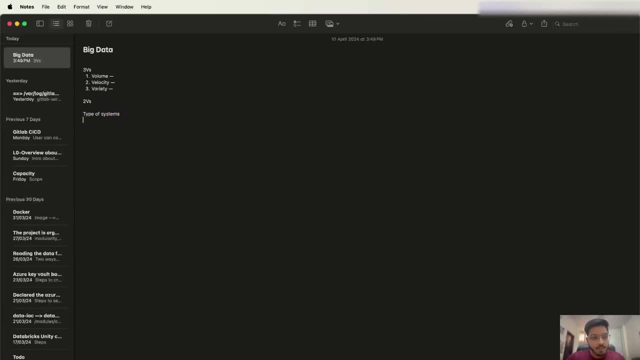 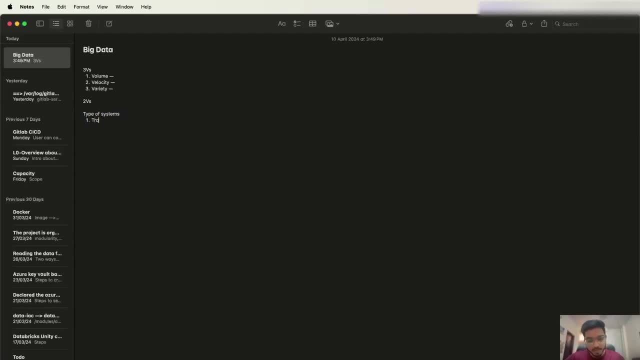 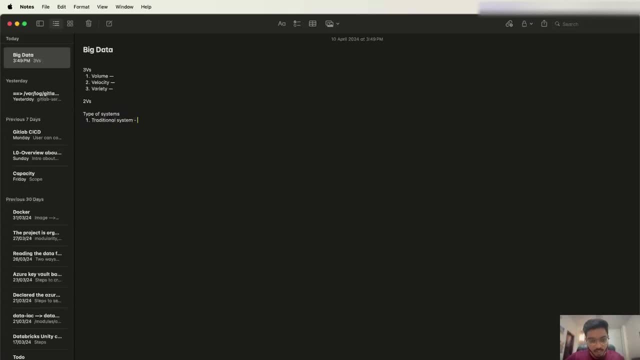 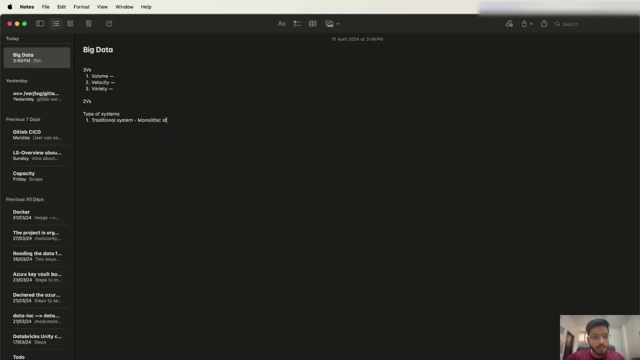 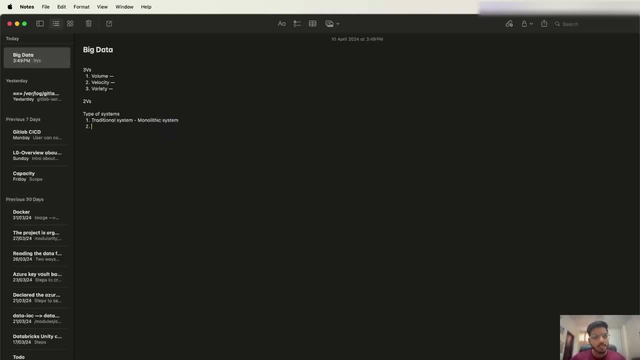 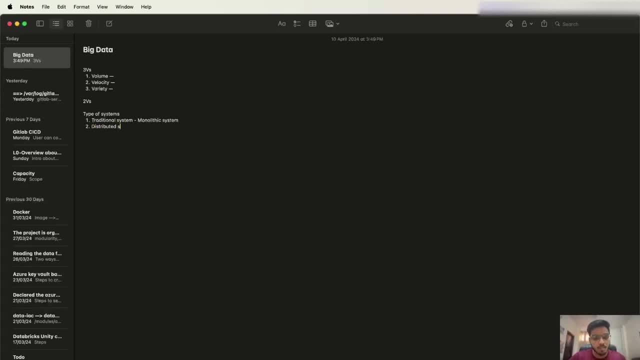 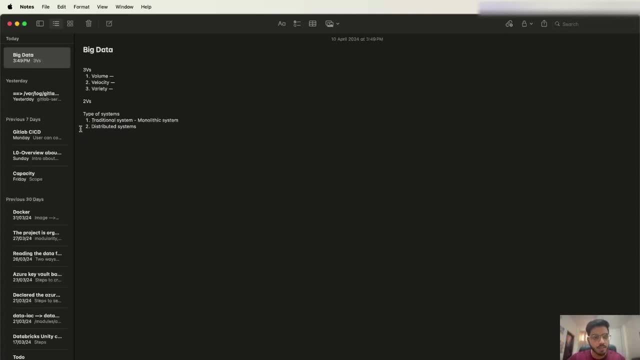 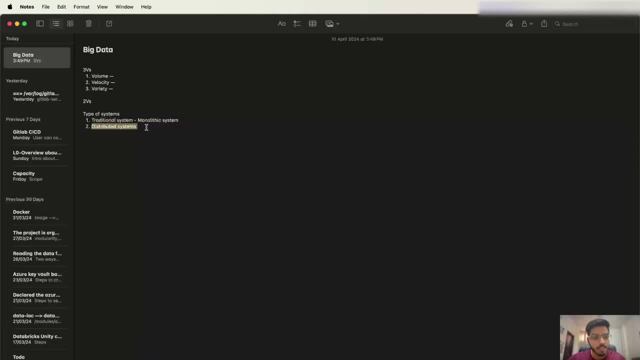 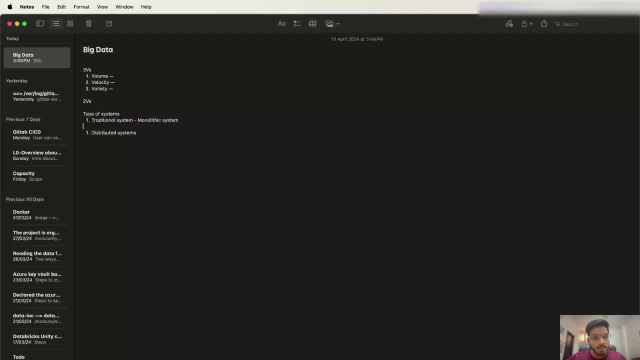 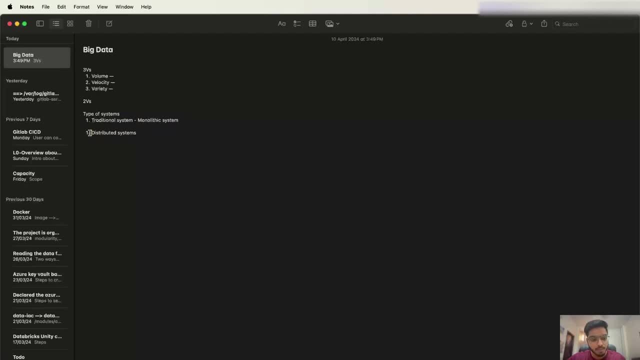 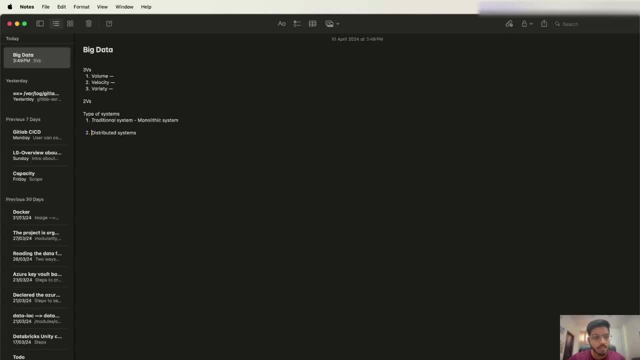 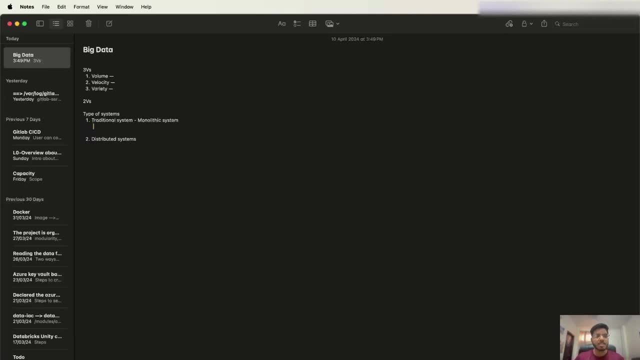 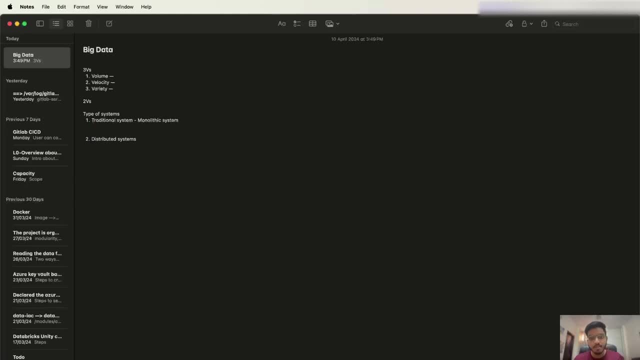 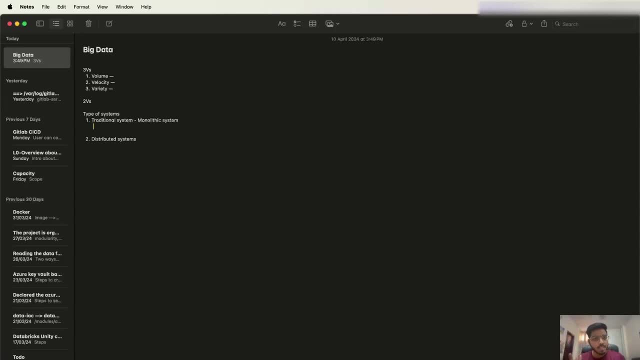 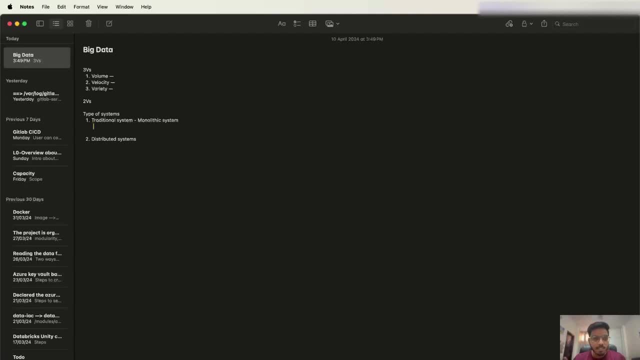 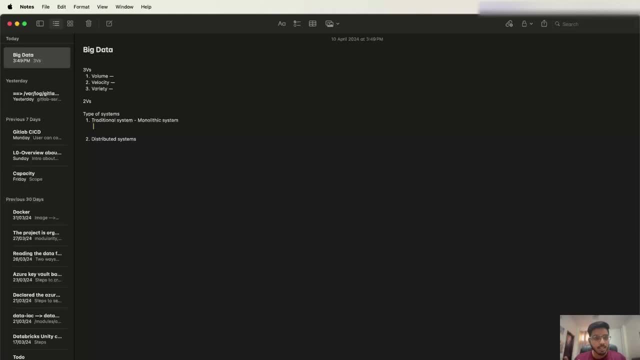 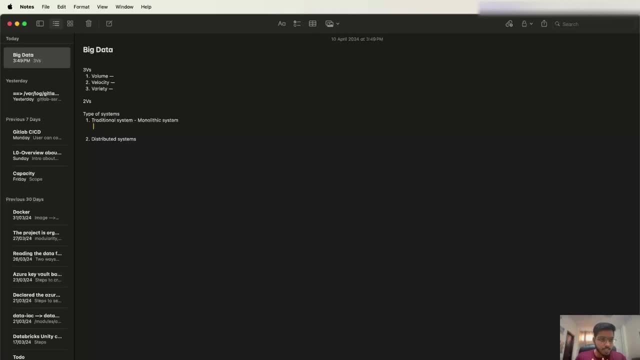 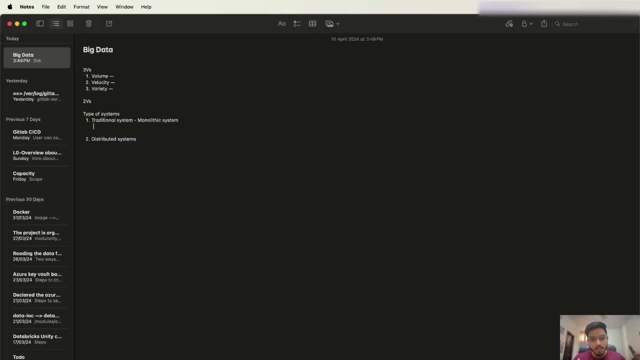 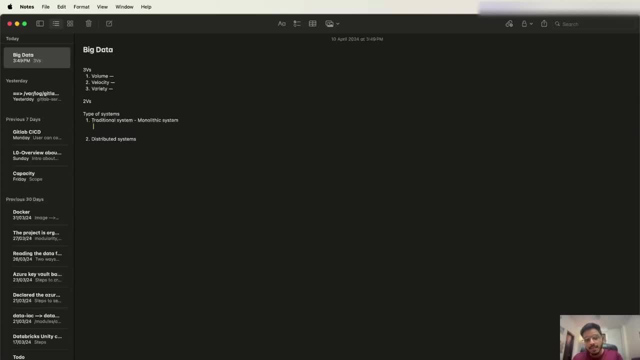 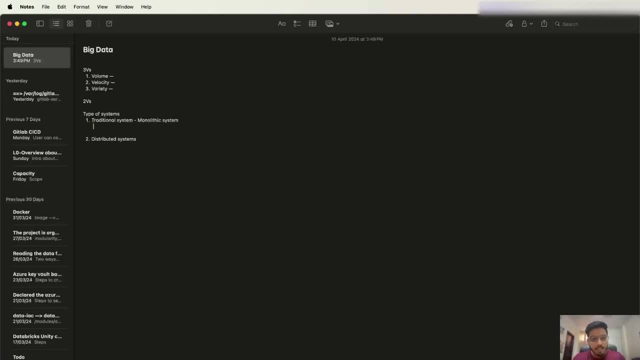 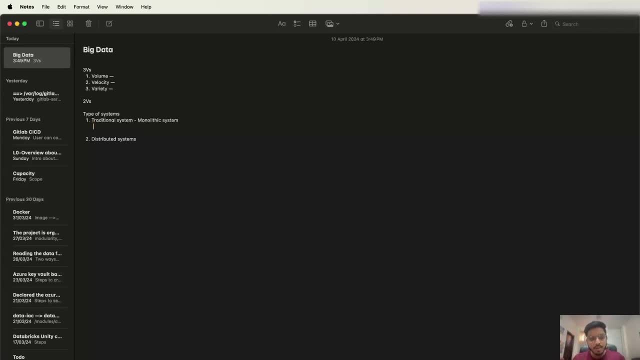 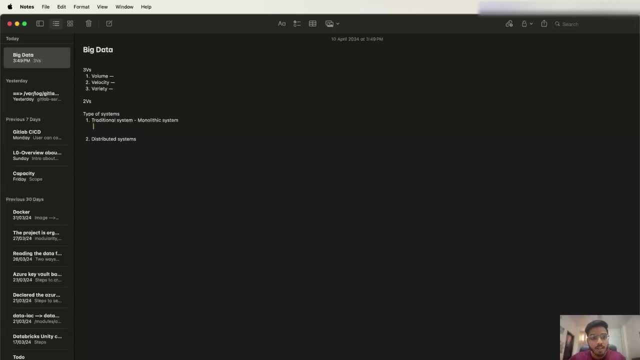 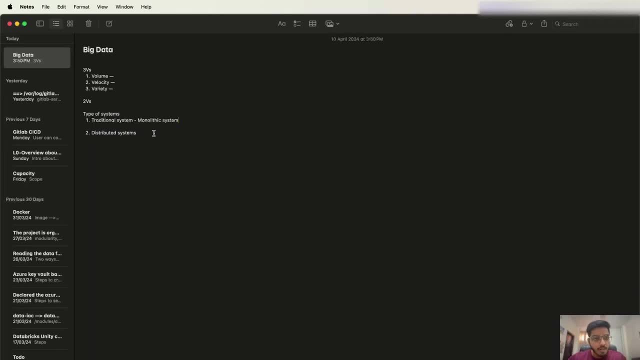 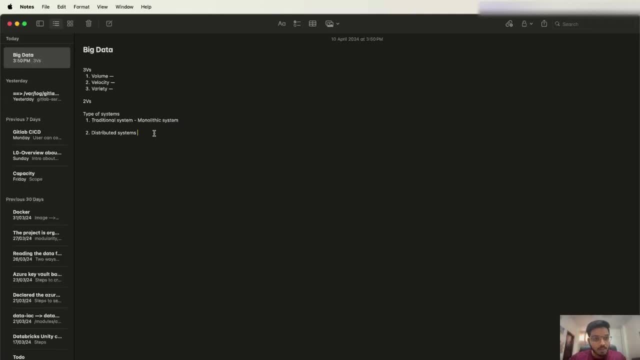 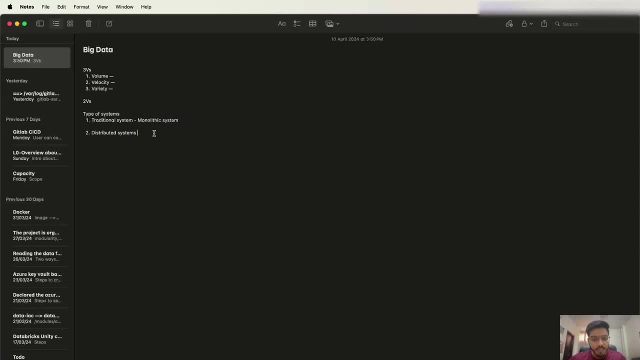 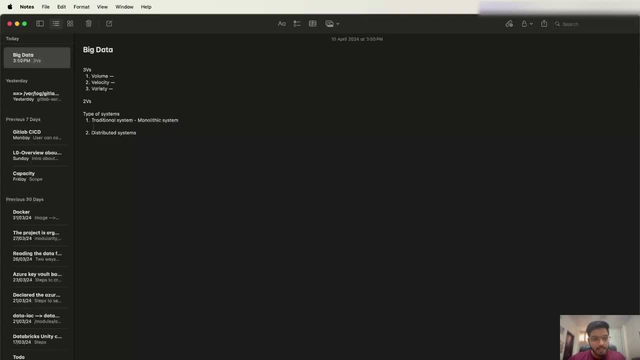 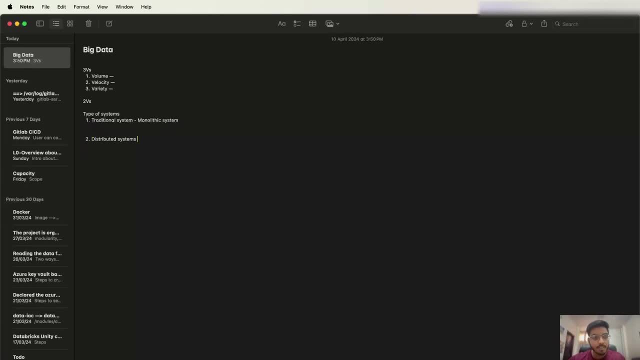 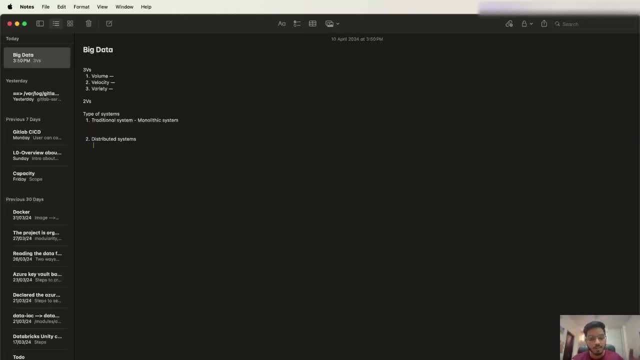 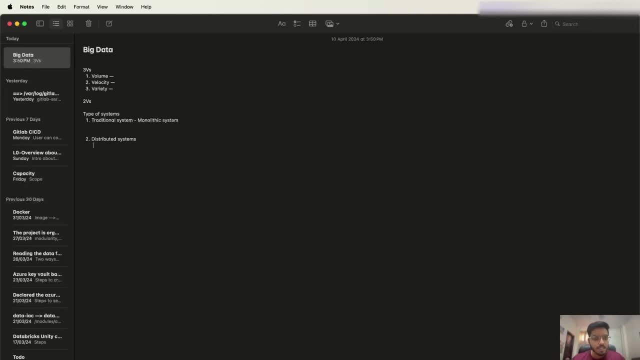 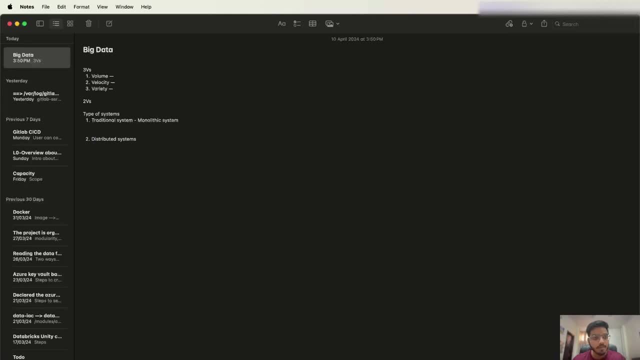 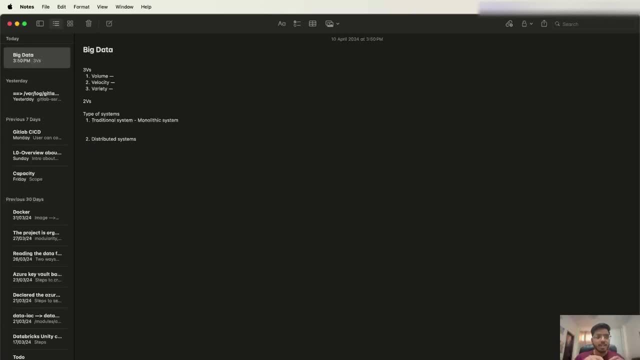 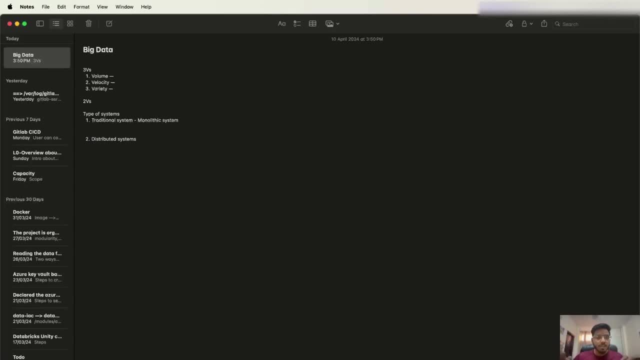 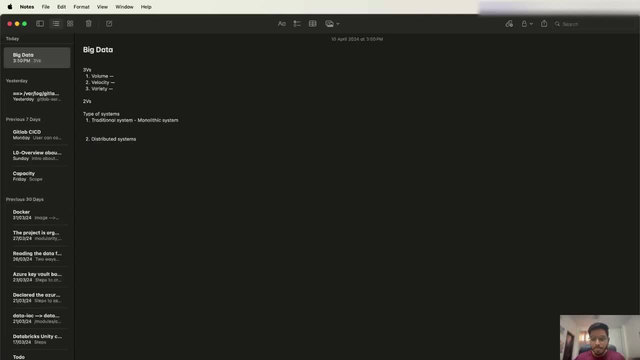 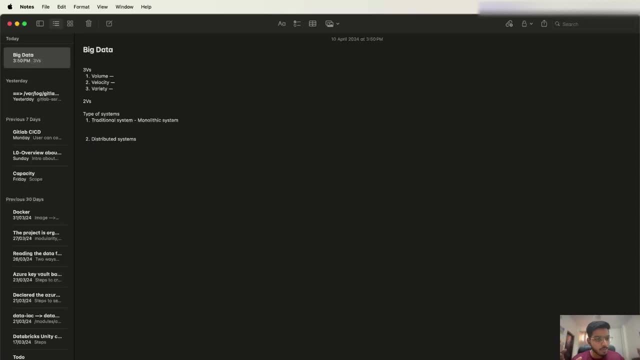 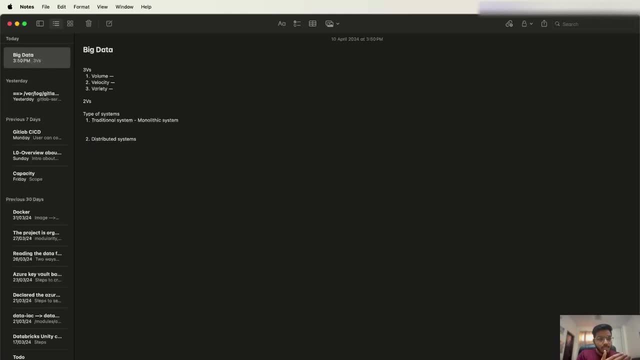 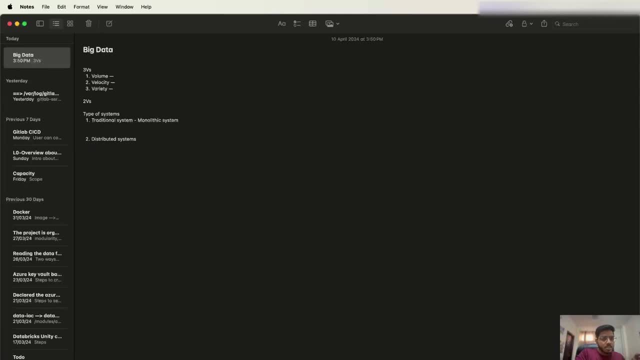 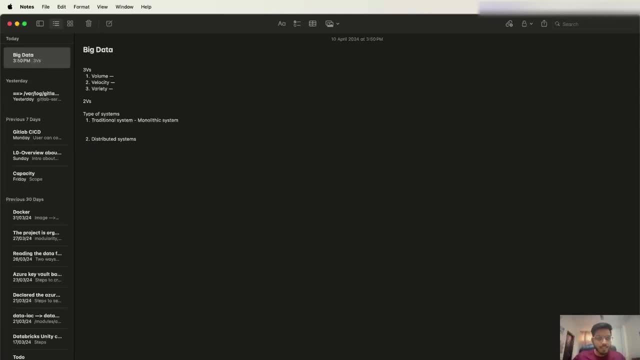 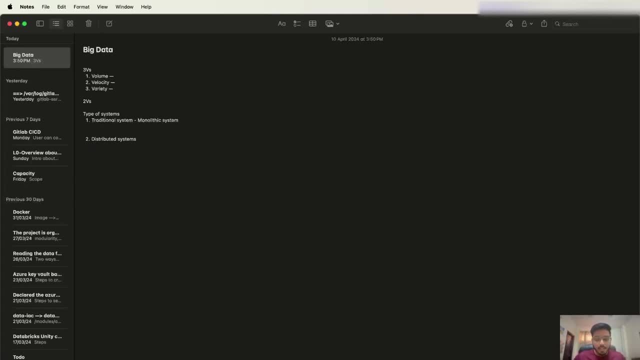 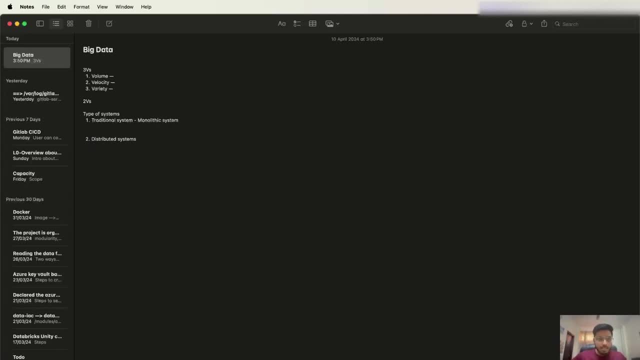 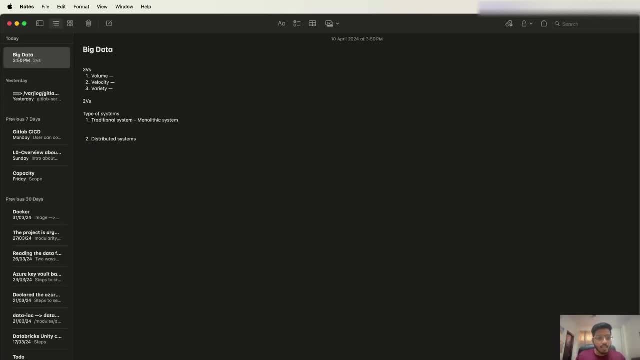 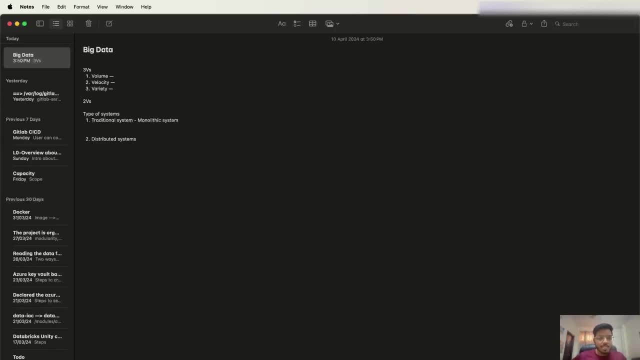 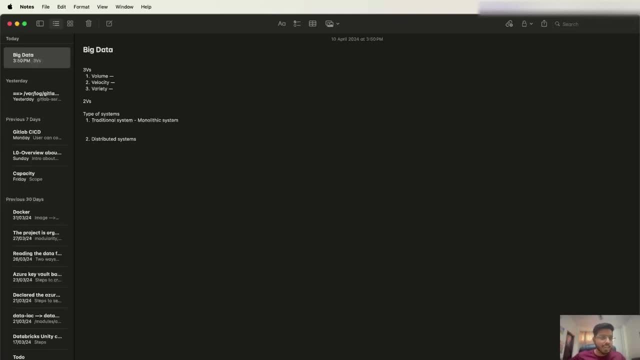 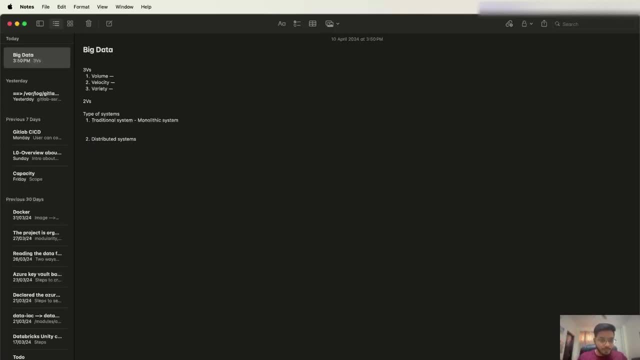 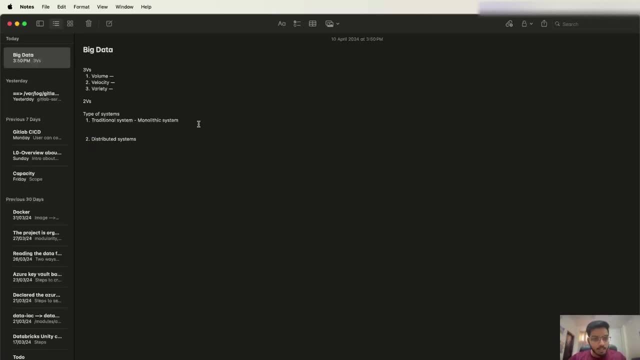 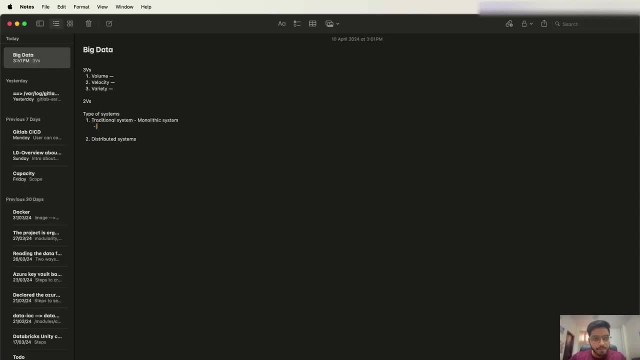 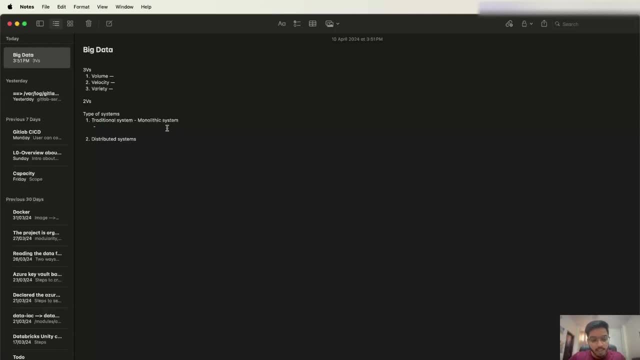 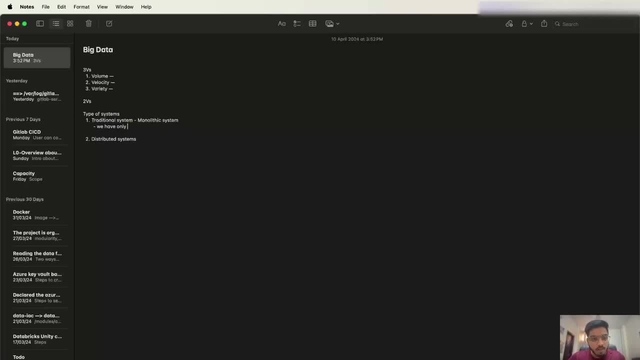 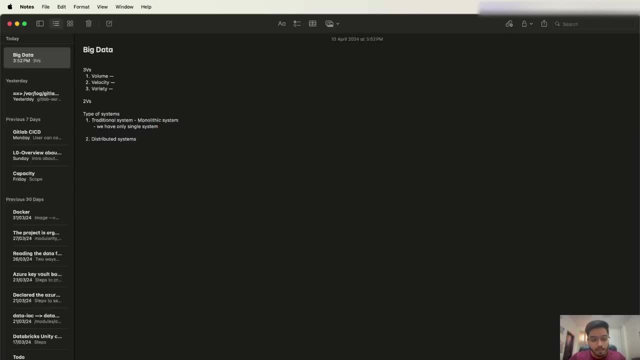 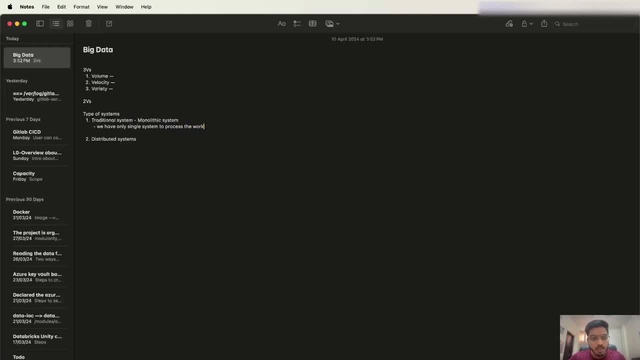 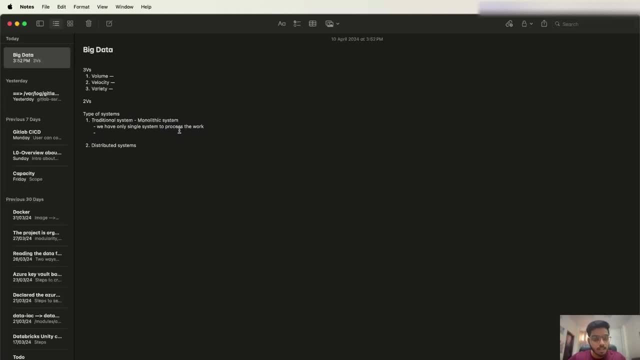 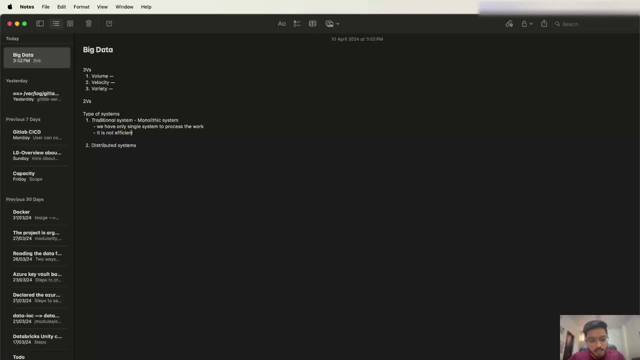 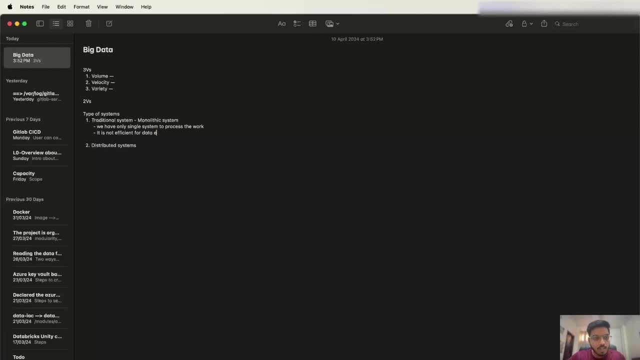 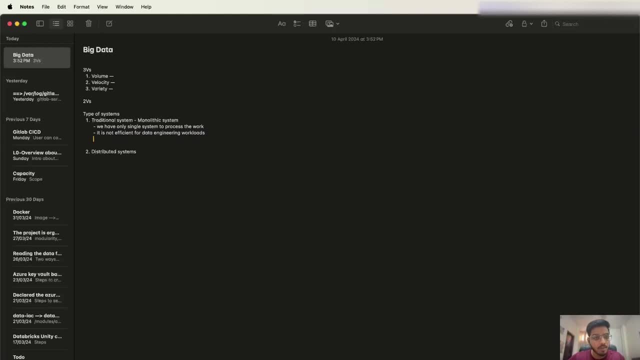 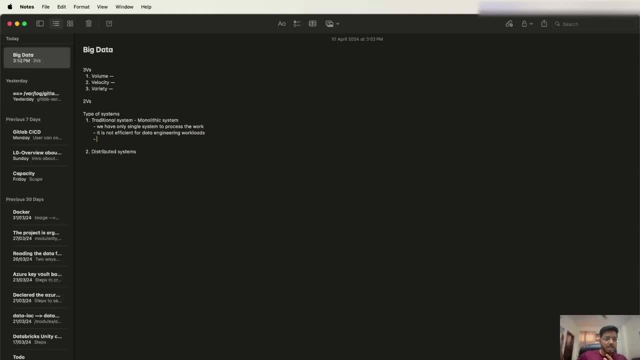 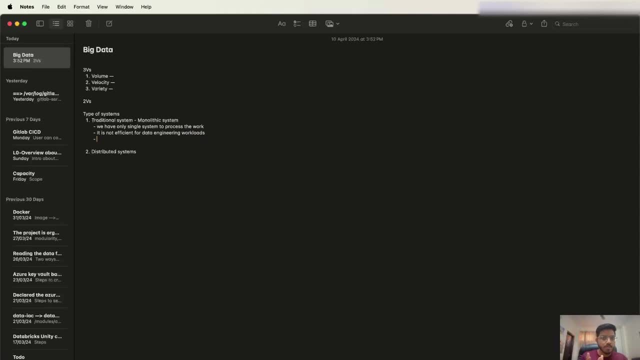 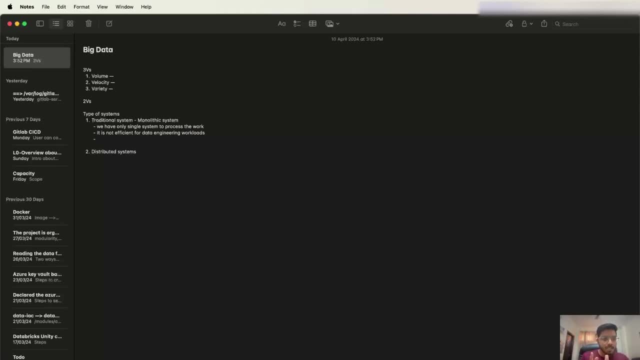 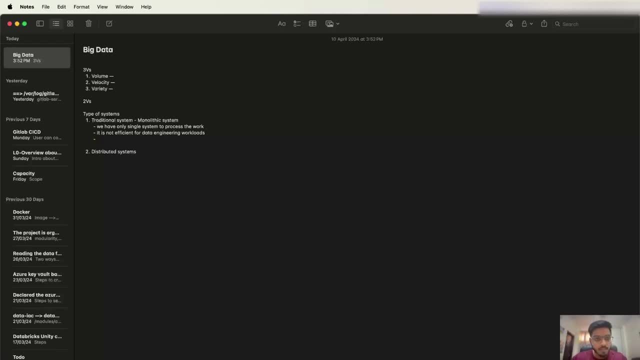 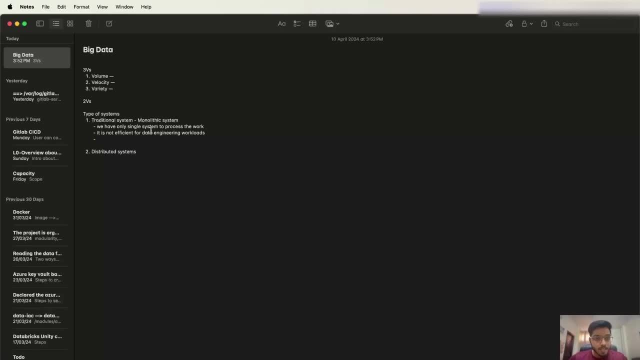 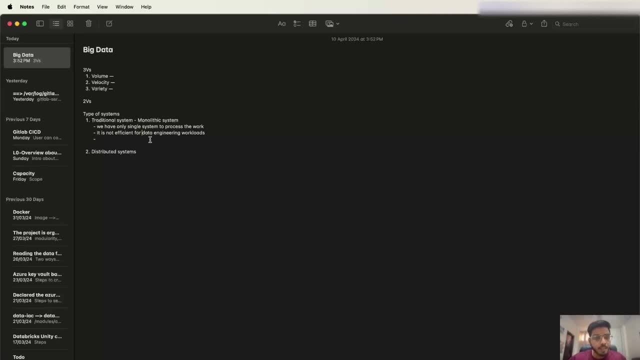 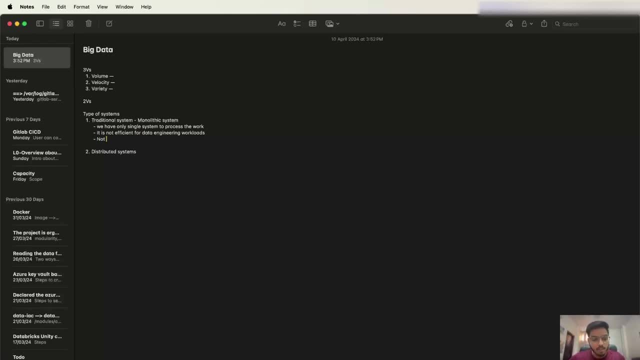 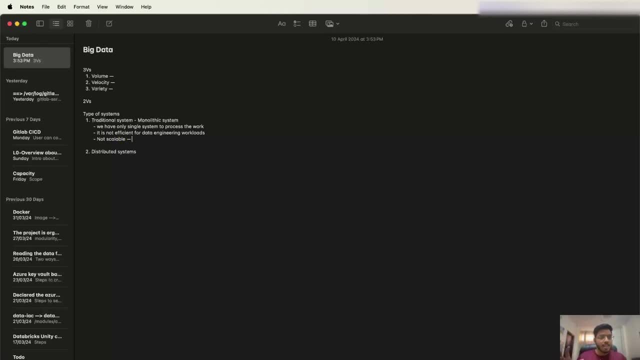 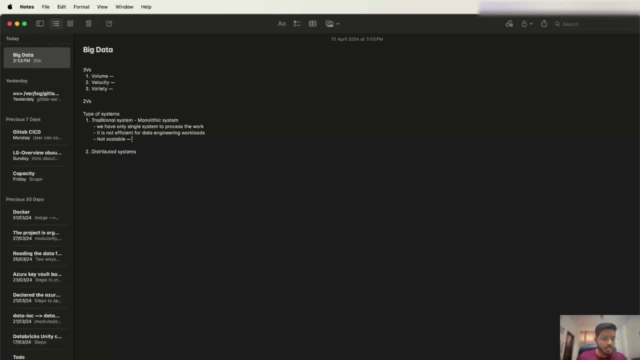 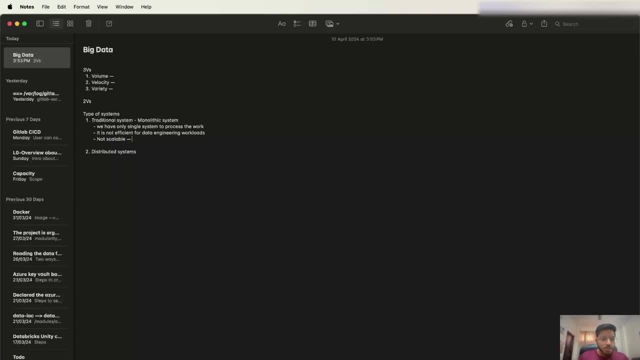 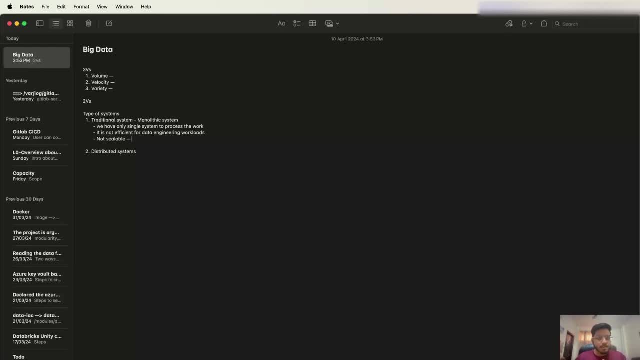 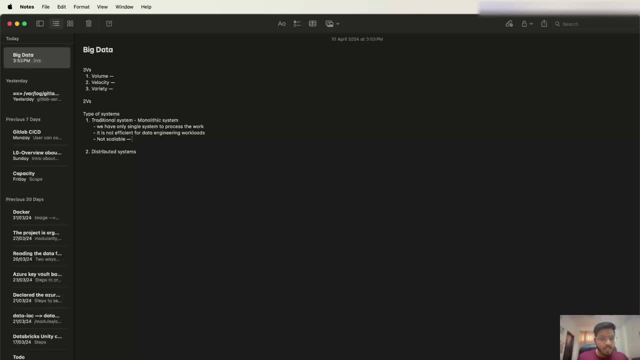 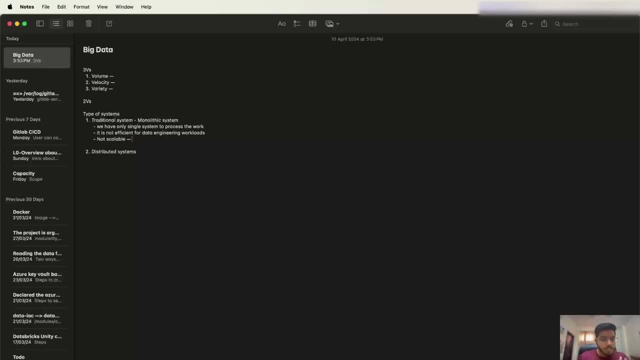 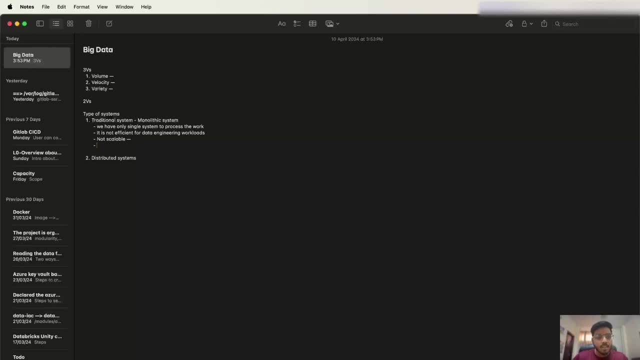 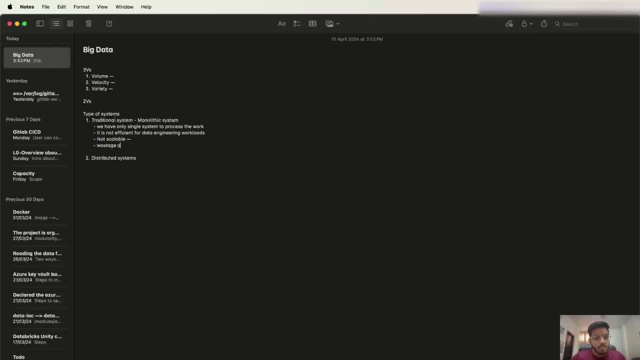 So velocity is nothing but the speed at which the data is coming. basically wastage of resources. what i mean by wastage of resources? suppose you are, you are getting, let's say, 10 gb data in your single system to get process and you added, and earlier you you. 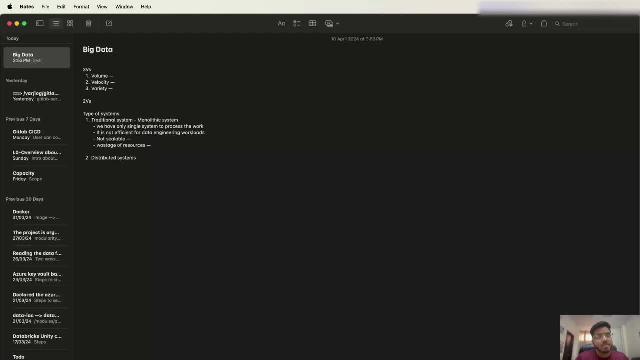 you had like say 5 gb ram only. so what you did is okay, i'll you have added, let's say, 20 gb ram, more 20, 20 more gb ram into your system. so now you have 25 gb ram and you are able to process. 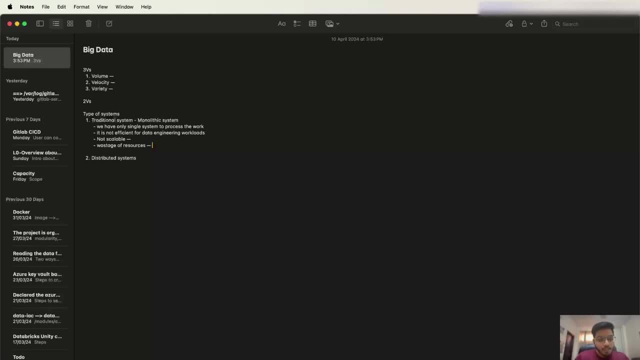 10 gb data very easily. but now what will happen next day? you start getting, let's say, 100 gb file, 100 gb file, okay. then you say, okay, i'll also again upgrade the ram to let's say, 150 gb ram. but what happens after that is the requirement changes and now you start getting 5 gb data only. 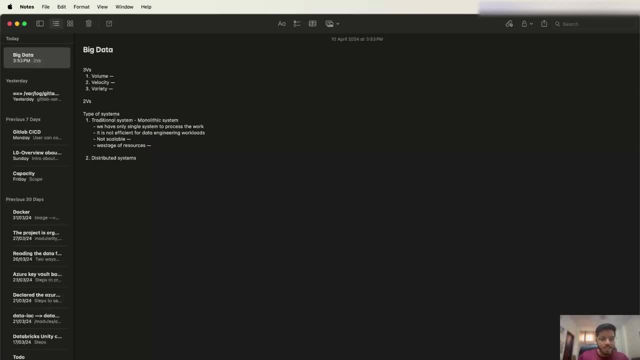 and so in this case, what will happen? you have increased your ram to 200 gb, but now you are only getting 5 gb ram, 5 gb data, so your 195 gb ram is unused and it will be like it will not be in use. uh. 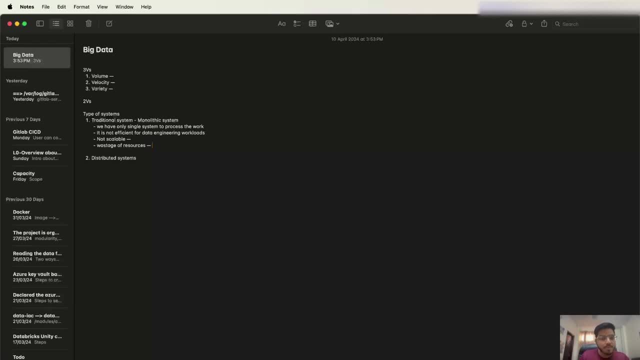 because you have. you have only 5 gb data that can be processed in, like, say, 5 to 10 gb ram. so then remaining ram is like waste and it is not being used for anything. so that is the wastage part, and yeah, so if i come to the distributed one. so so we can have multiple system, as i mentioned. 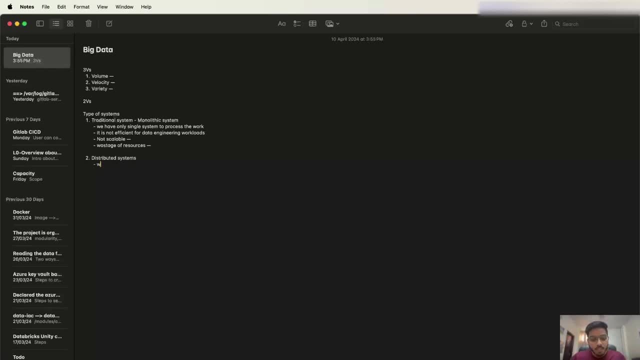 in the uh, the distributed system, so the work or the task will be distributed to the multiple machines. so okay, and it is very efficient for data engineering workloads because we can add any number of uh. uh, that is not basically. we can uh divide our data to different, to small chunks and process it? uh individually. 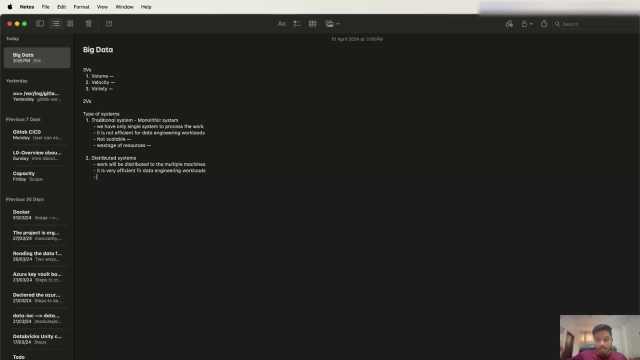 individually, like process uh, this small chunks on the uh multiple machine in a one go, like uh, and it will be very efficient and it will be completed in very less time compared to the single system, because now small chunks are processed and they add to parallelly these chunks are getting processed. 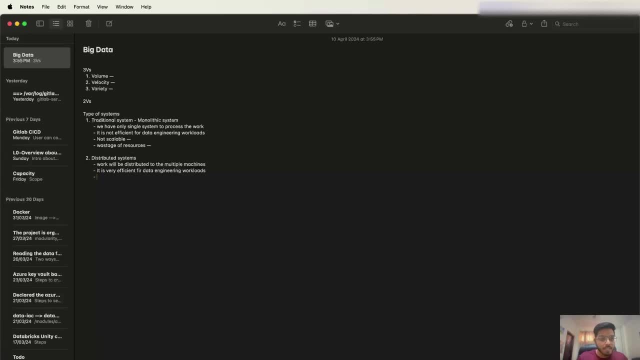 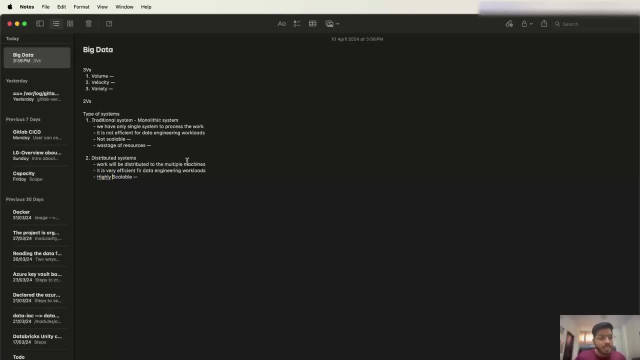 so it will be very efficient. and the scalable part- scalable part- is also like we: it is highly scalable. so it will be very efficient. and the scalable part- scalable part- is also like we. it is highly scalable because we can add any number of machines, any number of machines we can add in our network. there is no limit on that. 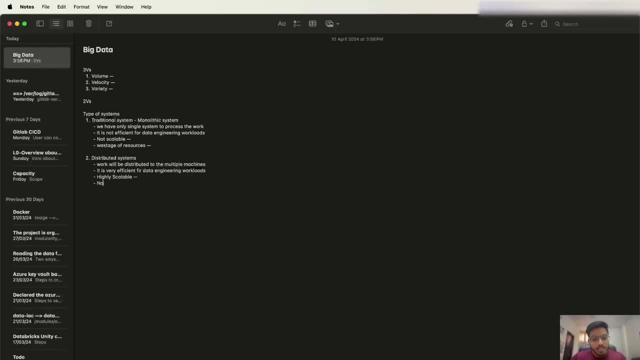 and so yeah, and no wastage, so let's move. so what you have understood is: uh, if we are using, we have to basically use the distributed systems to process the big data. distributed systems to process the big data, distributed systems to process the big data. so what? 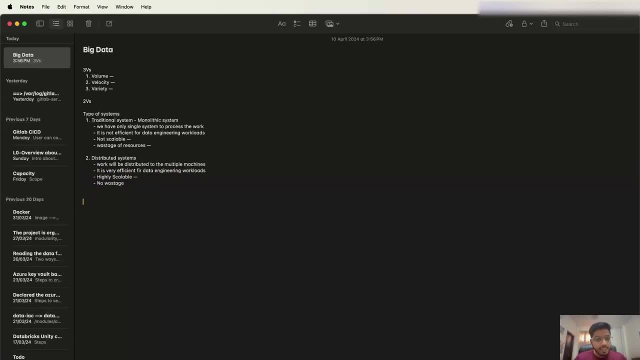 so what? so what is indirectly? it is saying like is indirectly. it is saying like is indirectly. it is saying like, at the end we will be building some data. at the end we will be building some data. at the end we will be building some data: big data application and. 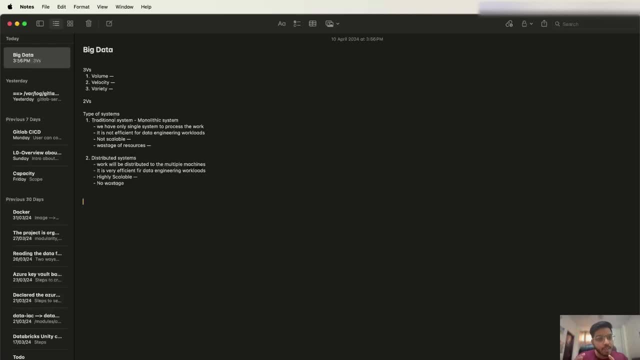 big data application and big data application, and we will be able to, we will be able to, we will be able to process the big data if we have the process, the big data, if we have the process, the big data, if we have the distributed system, distributed system. 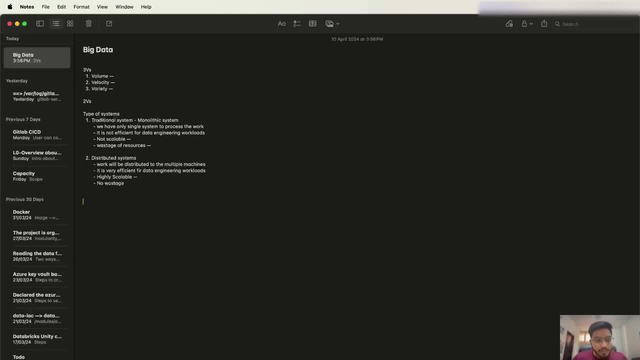 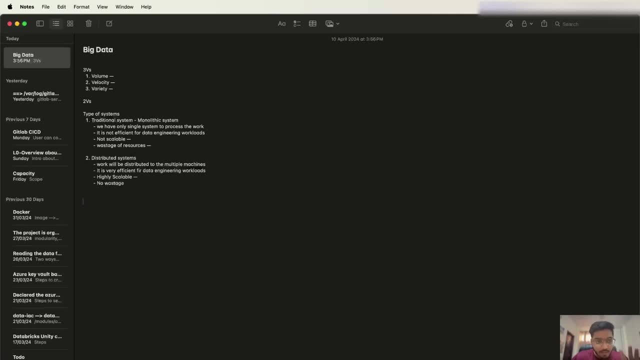 design a big data pipeline. so there are three things that we should, three things that we should, three things that we should consider, consider, consider before building any data pipeline: what is before building any data pipeline? what is before building any data pipeline? what is that is? that is. 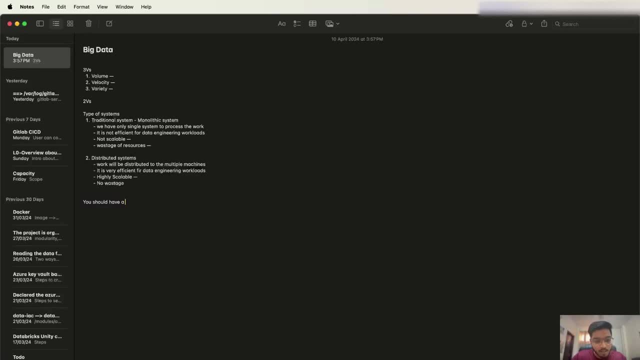 that is, you should have a scalable, scalable. scalable or not scalable, i would say, or not scalable, i would say: or not scalable. i would say: uh uh, uh. distributed, distributed, distributed storage, storage, storage, that should be scalable, that should be scalable, that should be scalable now, that should be scalable now. and another thing is: you should 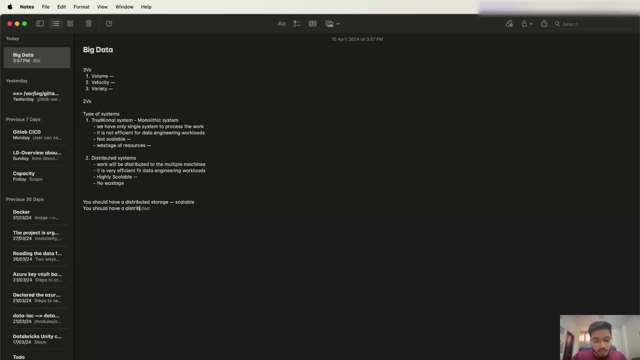 and another thing is you should, and another thing is you should have a, have a, have a distributed, distributed, distributed processing, processing, processing system, system, system, or i would say, or i would say, or i would say engine, engine, engine, and that has to be scalable. and if these first two things, uh, you, 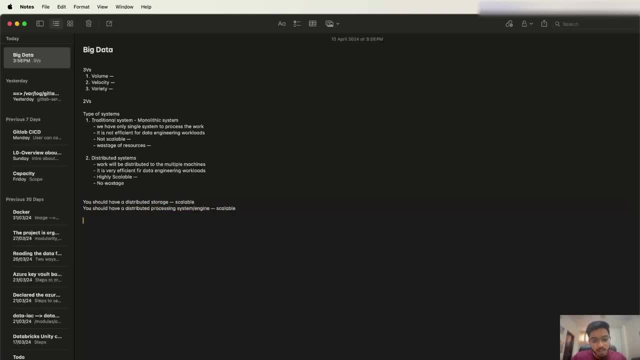 and if these first two things, uh, you, and if these first two things, uh, you somehow able to get, then your somehow able to get, then your somehow able to get, then your, then only your, then only your, then only your big data application will be scalable, will be scalable. 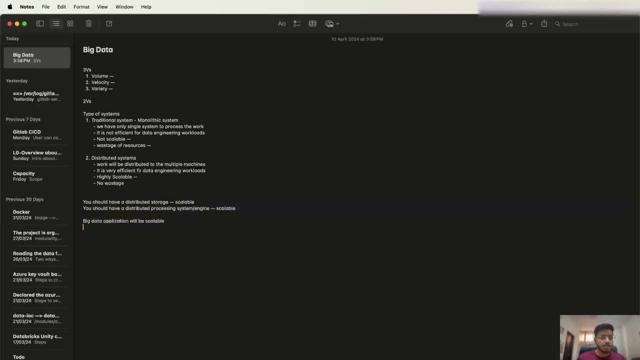 will be scalable. okay, so, these are the three things that okay. so, these are the three things that okay. so these are the three things that you have to, you have to, you have to take care about uh like, take care about, uh like, take care about uh like, while building your data platform, data. 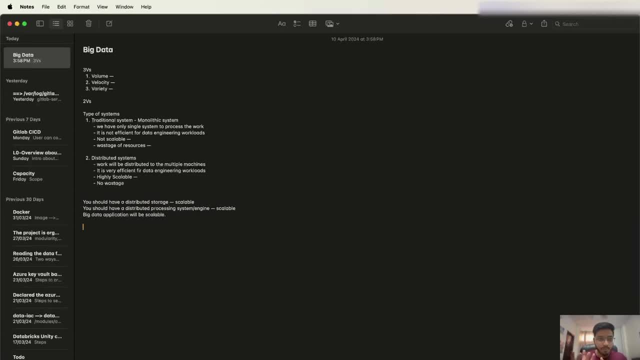 while building your data platform data, while building your data platform data big data application. basically so you, big data application. basically so you, big data application. basically so you should have a, should have a, should have a scalable distributed storage and that scalable distributed storage and that scalable distributed storage and that can handle any amount of data that can. 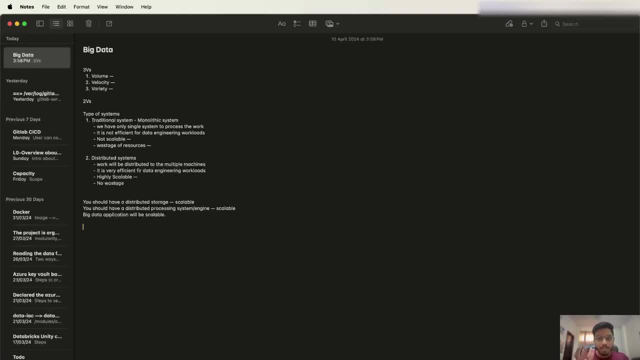 can handle any amount of data that can can handle any amount of data that can be scaled to any level, be scaled to any level, be scaled to any level. and you also have a distributed system. and you also have a distributed system. and you also have a distributed system because now you have connected your 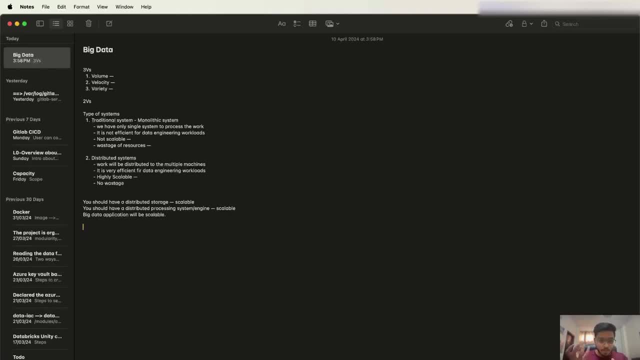 because now you have connected your, because now you have connected your multiple machines to some network, so multiple machines to some network, so multiple machines to some network. so there has to be some, there has to be some, there has to be some processing engine that will be processing. 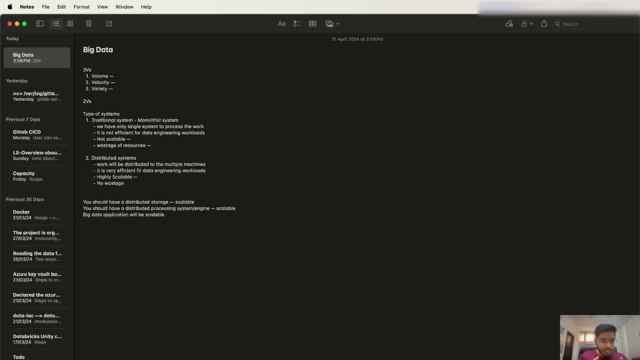 processing engine that will be processing processing engine that will be processing these, these, these small chunks of data on these multiple small chunks of data, on these multiple small chunks of data on these multiple machines. so there has to be some program machines, so there has to be some program. 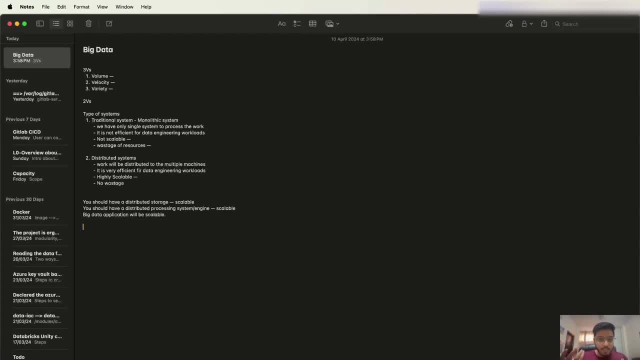 machines. so there has to be some program that will be doing this for you, that will be doing this for you, that will be doing this for you. so that has to be there, and then only so that has to be there, and then only so that has to be there, and then only of big data, how we should define the big. 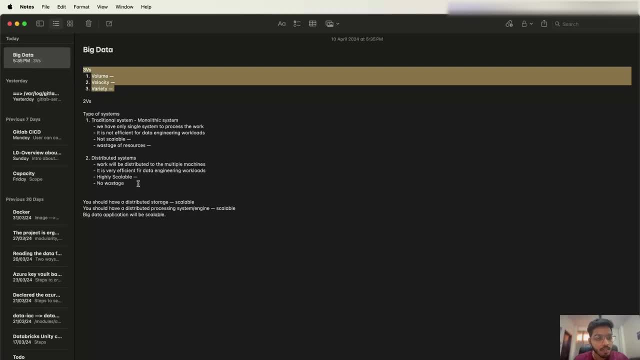 of big data, how we should define the big of big data, how we should define the big data. what is big data? and we also see data. what is big data? and we also see data. what is big data? and we also see. we saw that: uh, what kind of systems that. 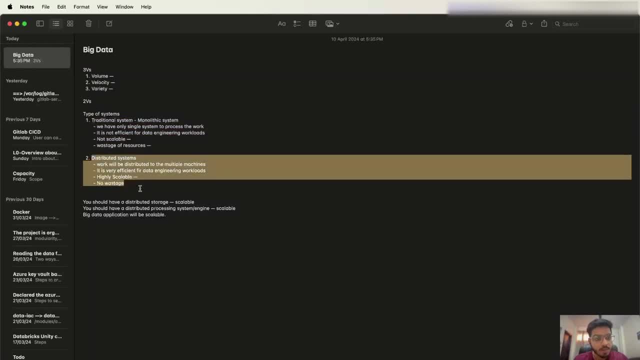 we saw that, uh, what kind of systems that. we saw that, uh, what kind of systems that are available and what kind of system are available and what kind of system are available and what kind of system that will help us to process a big data. that will help us to process a big data. 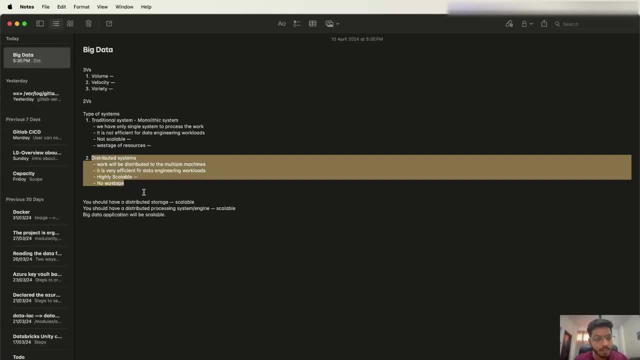 that will help us to process a big data and will help us to basically create a. and will help us to basically create a. and will help us to basically create a big data application or develop a big big data application, or develop a big big data application or develop a big data application. 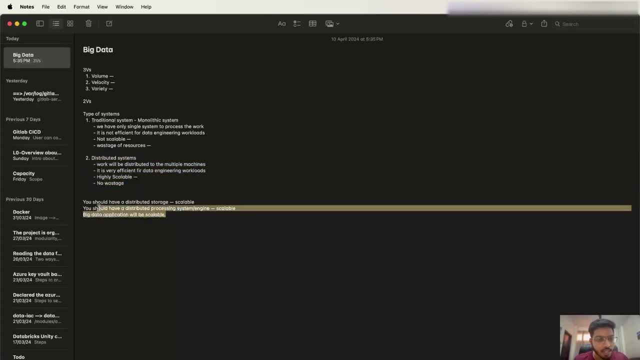 data application: data application. then we saw what, then we saw what, then we saw. what are the things that we should consider? are the things that we should consider, are the things that we should consider before building a big data application, before building a big data application, before building a big data application. and. 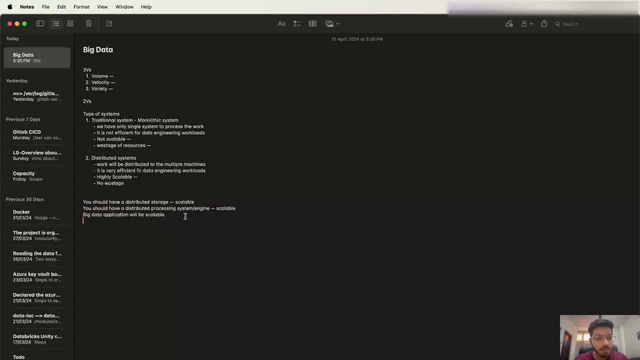 and and they will have like these things will. they will have like these things will they will have. like these things will help us in building a really scalable, help us in building a really scalable. help us in building a really scalable big data application. big data application, big data application. so, uh, till now, what we have discussed is: 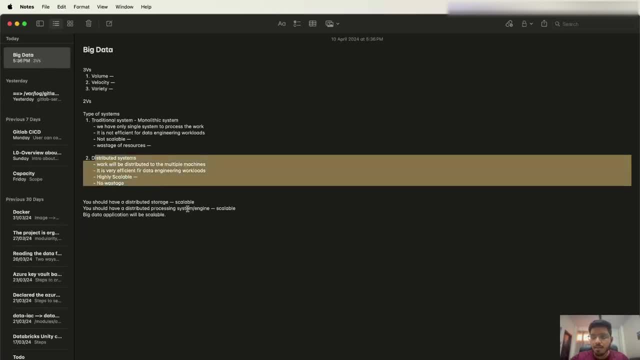 so uh, till now, what we have discussed is so uh, till now, what we have discussed is basically uh systems, basically uh systems, basically uh systems. that is nothing but uh. i would say a that is nothing but uh. i would say a that is nothing but uh. i would say a physical entity. 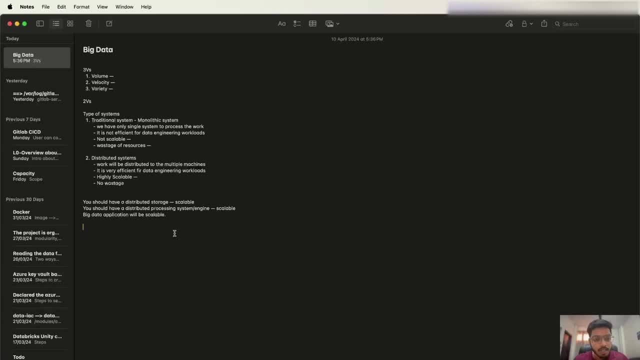 physical entity, physical entity systems are nothing, but the physical systems are nothing, but the physical systems are nothing but the physical thing, thing, thing. and so now let's move ahead and look at. and so now let's move ahead and look at. and so now let's move ahead and look at. what are the 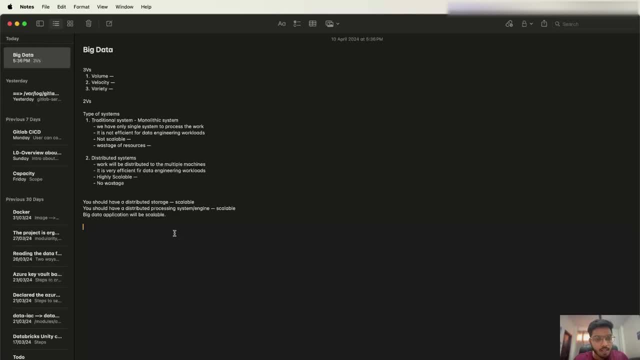 what are the? what are the frameworks? are there? what are the frameworks are there? what are the frameworks are there? what are the programs? programs? programs are there that will be installed on this? are there that will be installed on this? are there that will be installed on this system and using those? 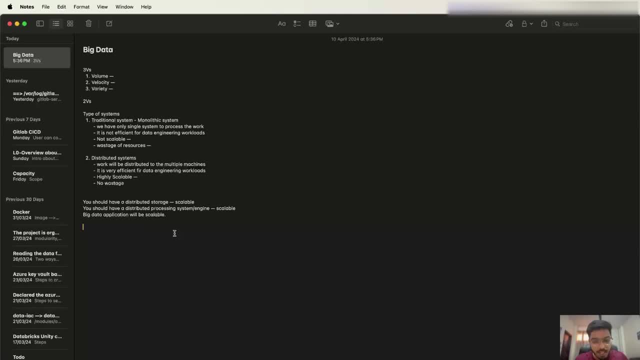 system and using those system and using those tools or frameworks, we will be tools or frameworks. we will be tools or frameworks. we will be processing, our processing, our processing our basically big data. we will be analyzing basically big data. we will be analyzing basically big data. we will be analyzing big data. we will be. 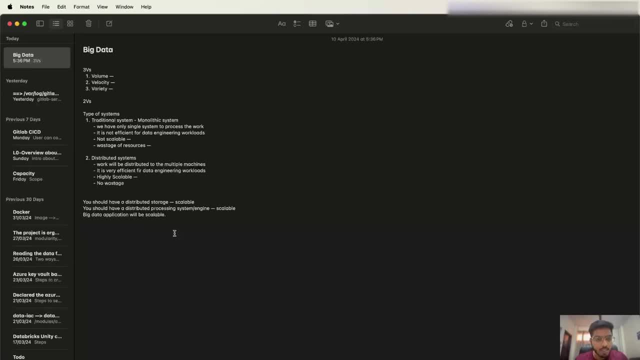 big data, we will be analyzing big data, we will be analyzing. so what are these tools and so what are these tools and so what are these tools and technologies? so the first technologies, so the first technologies. so the first thing is the hadoop you must have, thing is the hadoop you must have. 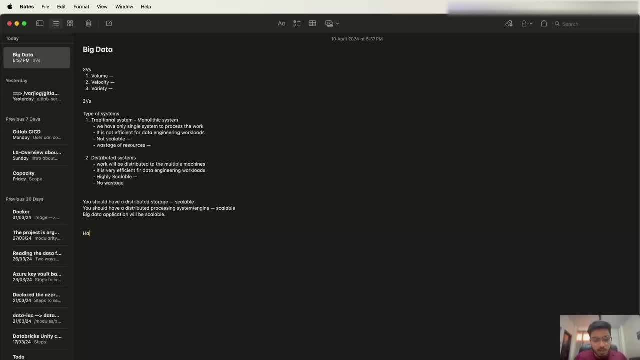 thing is the hadoop. you must have heard about hadoop in big data, heard about hadoop in big data, heard about hadoop in big data. so what is hadoop? so what is hadoop? so what is hadoop? for now, i will be giving very high level. 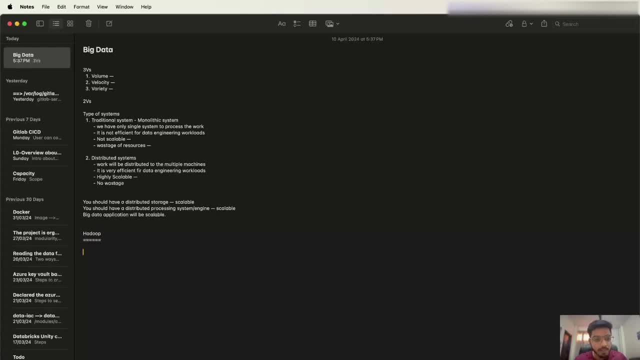 for now i will be giving very high level. for now i will be giving very high level overview and in the upcoming lectures we overview and in the upcoming lectures we overview and in the upcoming lectures we will go deep, dive into these, will go deep, dive into these. 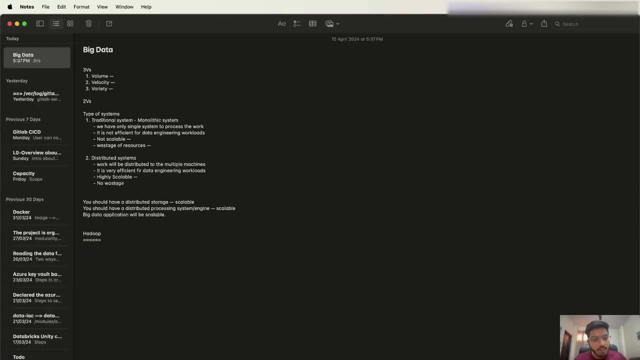 will go deep dive into these. hadoop spark very deep dive, okay. so hadoop spark very deep dive, okay. so hadoop spark very deep dive, okay. so for now, let's just uh look at this. so for now, let's just uh look at this. so for now, let's just uh look at this. so in hadoop, hadoop is nothing but a. 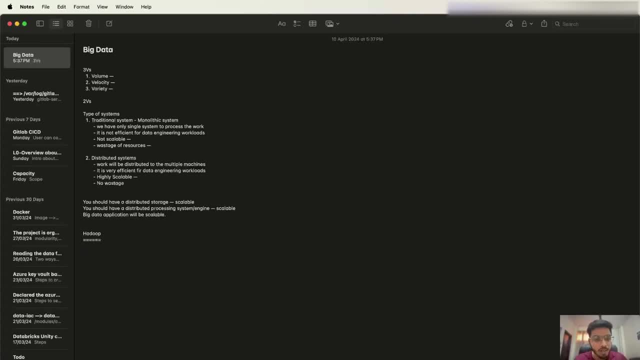 in hadoop. hadoop is nothing but a in hadoop. hadoop is nothing but a ecosystem. it is not a specific tool. ecosystem: it is not a specific tool. ecosystem: it is not a specific tool. hadoop is not a tool. hadoop is an. hadoop is not a tool. hadoop is an. 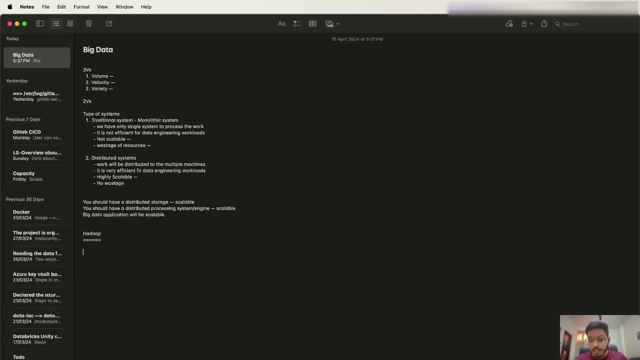 hadoop is not a tool. hadoop is an ecosystem of tools, for example: uh, ecosystem of tools, for example, uh, ecosystem of tools, for example, uh, i'll give it an example- is: let's say- i'll give it an example- is, let's say- i'll give it an example, is, let's say we have apple, we. we generally say like: 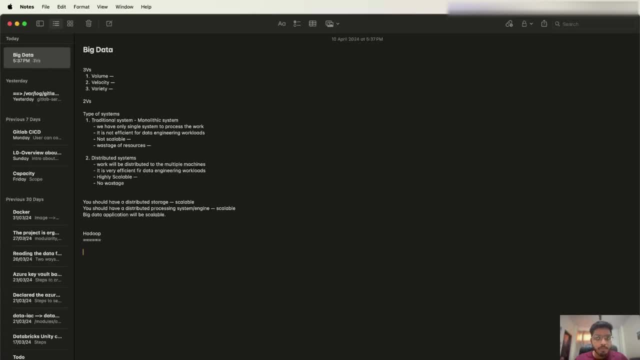 we have apple. we we generally say: like we have apple. we we generally say: like apple has a very good ecosystem, what apple has a very good ecosystem, what apple has a very good ecosystem. what does it mean: like apple, we have apple. does it mean: like apple, we have apple? 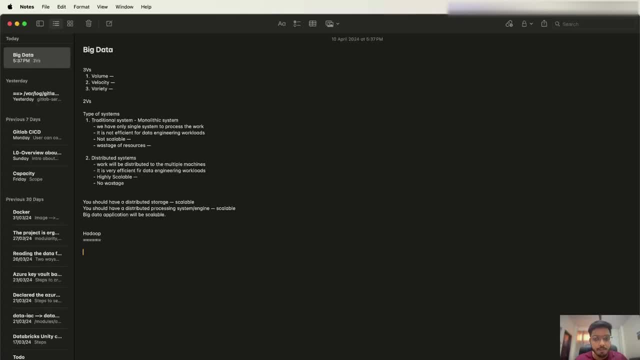 does it mean, like apple, we have apple watch, we have apple macbook laptop, we watch. we have apple macbook laptop, we watch. we have apple macbook laptop. we have apple's ipad. we have apples. you have apple's ipad. we have apples. you have apple's ipad. we have apples. you know phone. 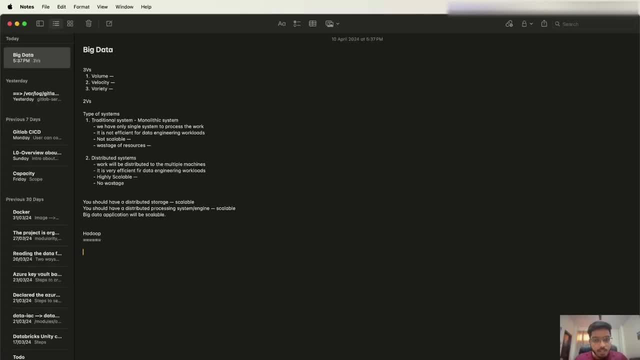 know phone, know phone airpods, etc. the internally the core airpods, etc. the internally the core airpods etc. the internally the core machine, basically, machine, basically machine. basically the chips are developed by apple only. so the chips are developed by apple only, so the chips are developed by apple only so the core part is same in all these. 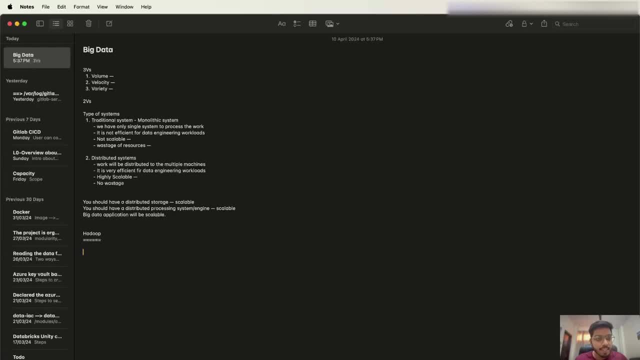 the core part is same in all these. the core part is same in all these: uh basically tech, uh in these devices, uh basically tech, uh in these devices, uh basically tech, uh in these devices. and they are interlinked and so, and they are interlinked and so. 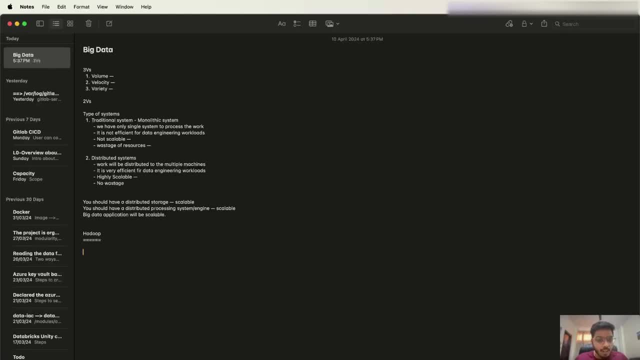 and they are interlinked and so, basically these devices are catering to, basically these devices are catering to. basically these devices are catering to different use cases, different use cases, different use cases, basically like phone. you are using for a. basically like phone. you are using for a. basically like phone. you are using for a different purpose, laptop using. you are 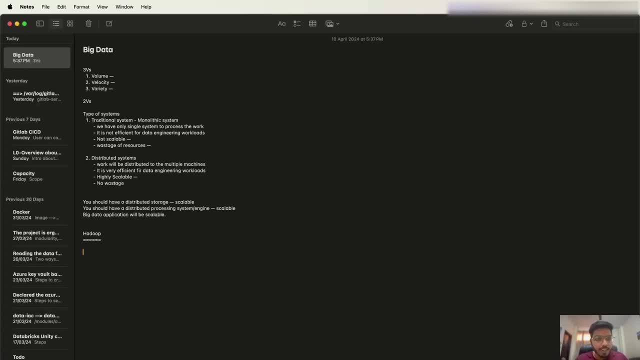 different purpose. laptop using you are different purpose. laptop using you are using for a different, different purpose, using for a different, different purpose, using for a different, different purpose. but the core functionality, but the core, but the core functionality, but the core, but the core functionality, but the core thing that is being used in these. 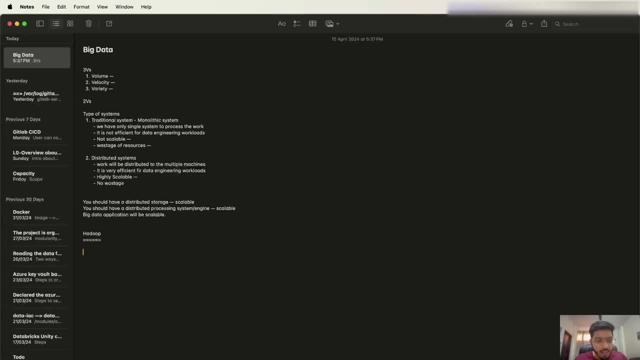 thing that is being used in these, thing that is being used in these devices are same. that are developed by devices are same. that are developed by devices are same that are developed by the apple, the apple, the apple. on this, and if you look at the hadoop, 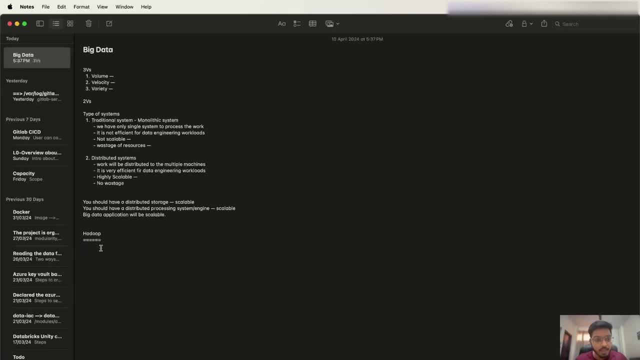 on this, and if you look at the hadoop on this, and if you look at the hadoop ecosystem, ecosystem, ecosystem. so i'm just trying to relate so that you, so i'm just trying to relate so that you, so i'm just trying to relate so that you will be able to remember these things. 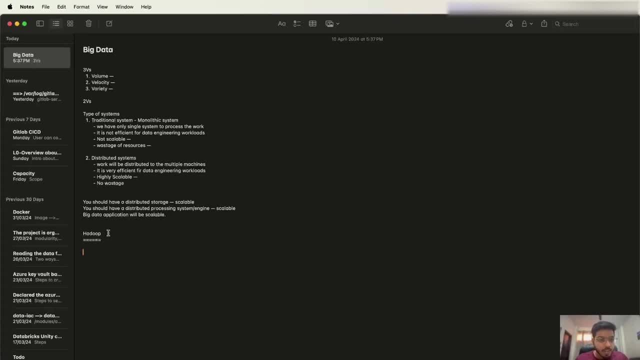 will be able to remember these things, will be able to remember these things and do not have to. you know, mug up the and do not have to. you know, mug up the and do not have to. you know, mug up the things. so in hadoop, hadoop has a ecosystem. 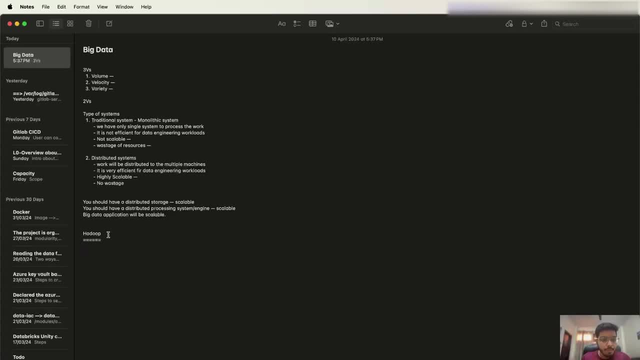 things. so in hadoop, hadoop has a ecosystem. things. so in hadoop, hadoop has a ecosystem. hadoop is an ecosystem. it has a number of. hadoop is an ecosystem, it has a number of. hadoop is an ecosystem. it has a number of catering to different use cases. so hadoop- 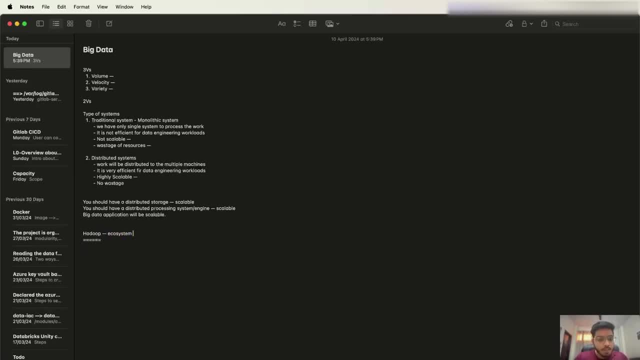 catering to different use cases. so hadoop catering to different use cases. so hadoop is nothing but is nothing but is nothing but a ecosystem. and the core components: uh, there are three core components. uh, there are three core components. uh, there are three core components basically. uh, in hadoop, uh, we have three. 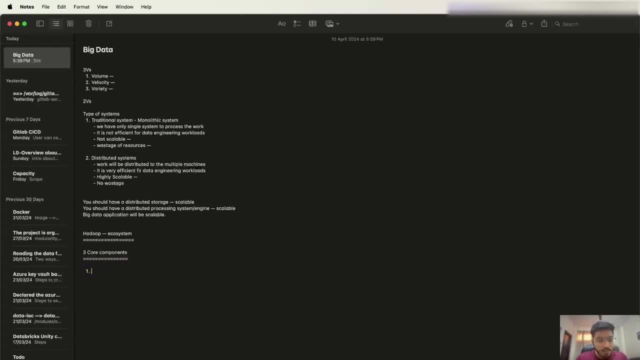 basically: uh in hadoop, uh, we have three. basically, uh in hadoop, uh, we have three, three core components and these core, three core components and these core three core components, and these core components are nothing but components are nothing, but components are nothing but first is sdfs, second is: 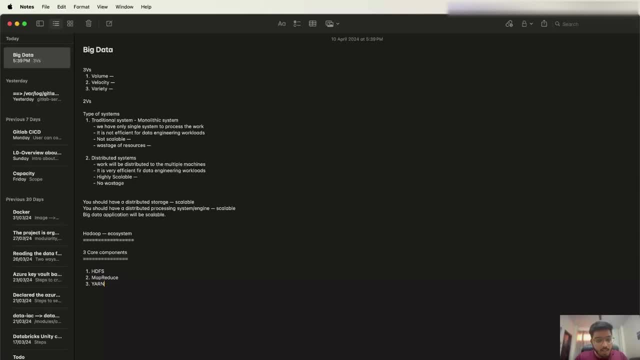 sdfs. second is sdfs. second is map, map, map, reduce, reduce, reduce. third is: third is: third is yarn. so let's see these core components yarn. so let's see these core components yarn. so let's see these core components. so, uh, the first core component is sdfs. 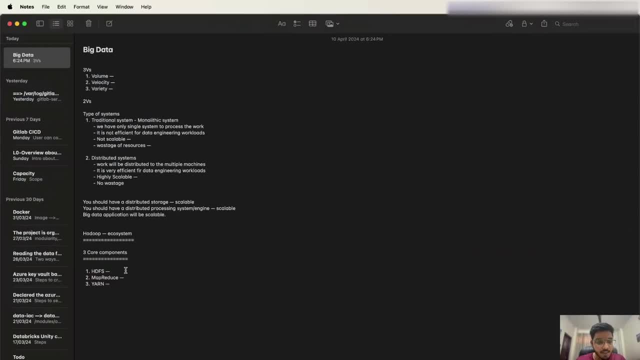 so, uh, the first core component is sdfs. so, uh, the first core component is sdfs. sdfs is nothing but hadoop. distributed sdfs is nothing but hadoop. distributed sdfs is nothing but hadoop. distributed file system, file system, file system. this will help us to store, manage our 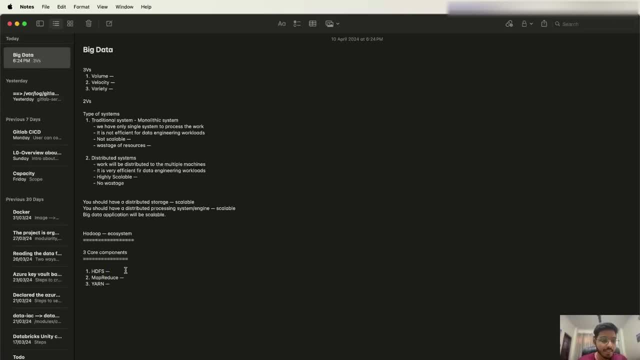 this will help us to store, manage our. this will help us to store, manage our, the data, the data we have, the data, the data we have, the data, the data we have on the distributed file system, on the, on the distributed file system, on the, on the distributed file system, on the distributed system. so we need some. 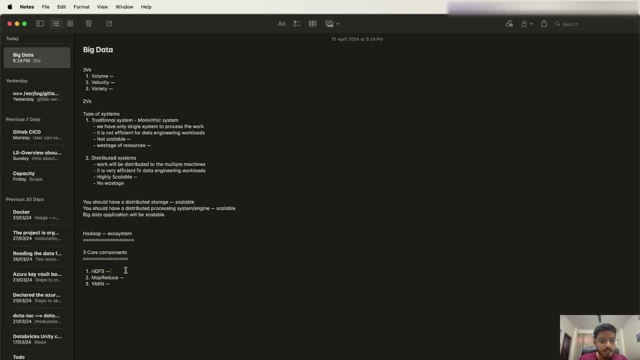 distributed system. so we need some distributed file system. so we need some file system that will help us to manage file system that will help us to manage file system that will help us to manage, store the data on these machines on the. store the data on these machines on the. 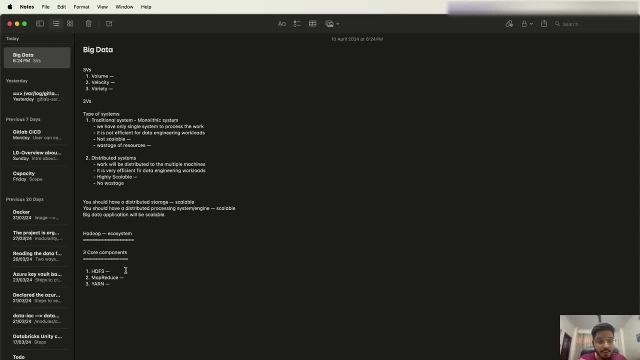 store the data on these machines, on the distributed system. distributed system, distributed system: basically, we need some file system. that basically we need some file system. that basically we need some file system that will manage our data, that will manage our data, that will manage our data, that will help us to store our data. okay, so, 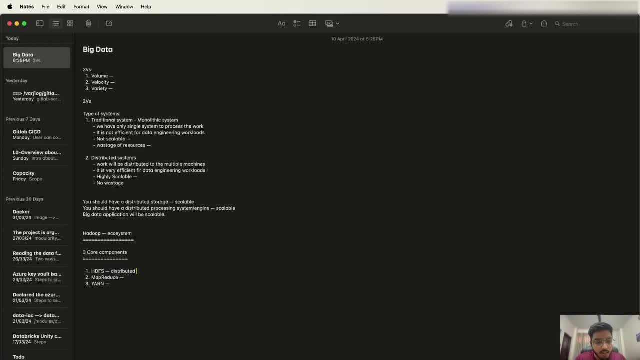 will help us to store our data, okay. so will help us to store our data, okay. so this is a distributed, this is a distributed, this is a distributed file system. you can say: or a storage file system. you can say: or a storage file system. you can say: or a storage. for a simplicity. 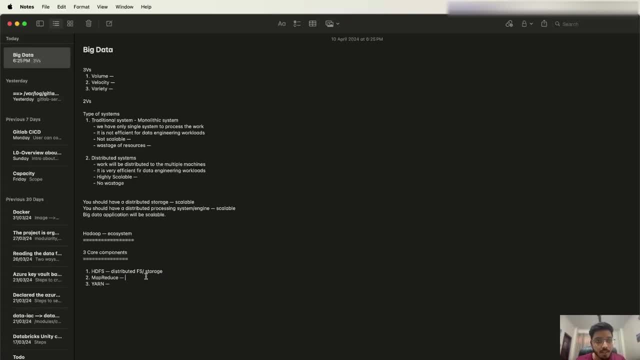 and then we have a map reduce map, and then we have a map reduce map, and then we have a map reduce map. reduce is nothing but a distributed reduce is nothing but a distributed reduce is nothing but a distributed processing engine. uh, why i'm saying processing engine? uh, why i'm saying: 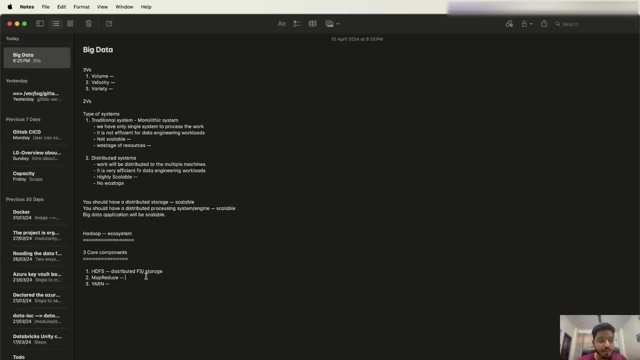 processing engine. uh, why i'm saying distributed processing? it is a basically distributed processing. it is a basically distributed processing. it is a basically processing engine, but it will processing engine, but it will processing engine. but it will, we will be using this processing engine. we will be using this processing engine. 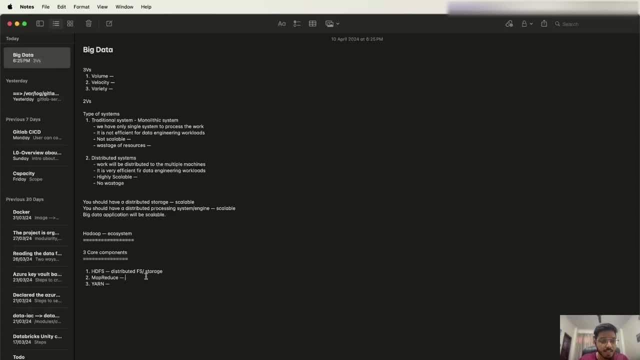 we will be using this processing engine on the distributed system. that's why we on the distributed system, that's why we on the distributed system, that's why we are saying this is a distributed, are saying this is a distributed, are saying this is a distributed processing engine. so this uh, 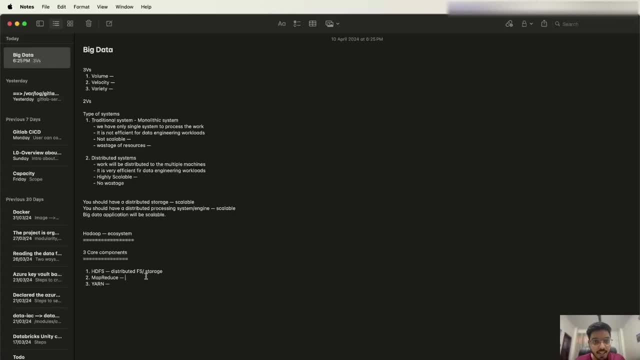 processing engine. so this uh processing engine, so this uh map reduce will basically help us to map reduce, will basically help us to map reduce, will basically help us to process our data in efficient way in an process, our data in efficient way in an process, our data in efficient way, in an efficient manner, so that we will be able 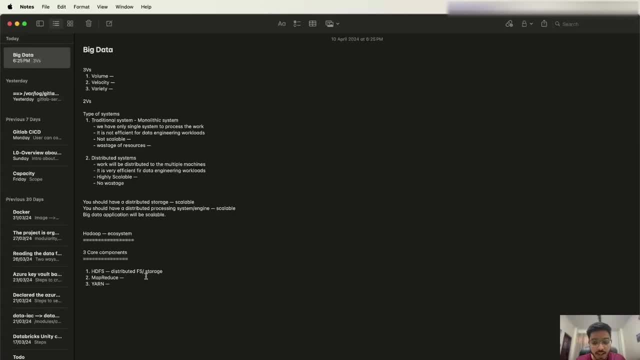 efficient manner so that we will be able, efficient manner so that we will be able to achieve some parallelism. we will be to achieve some parallelism. we will be to achieve some parallelism. we will be able to achieve the parallelism parallel, able to achieve the parallelism parallel. 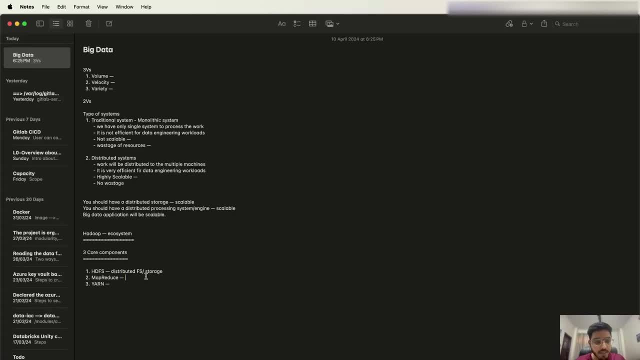 able to achieve the parallelism parallel processing that i'll be covering in the processing that i'll be covering in the processing that i'll be covering in the new uh upcoming lecture. what are the new uh upcoming lecture? what are the new uh upcoming lecture? what are the parallel parallelism? what is parallelism? 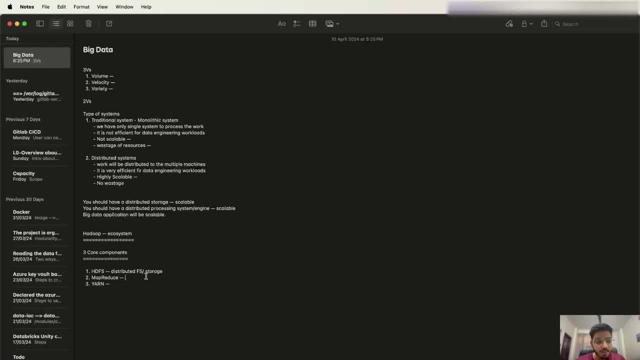 parallel parallelism. what is parallelism? parallel parallelism, what is parallelism? what is parallel processing? so that i'll what is parallel processing, so that i'll what is parallel processing, so that i'll cover. but for now just understand this cover, but for now just understand this. 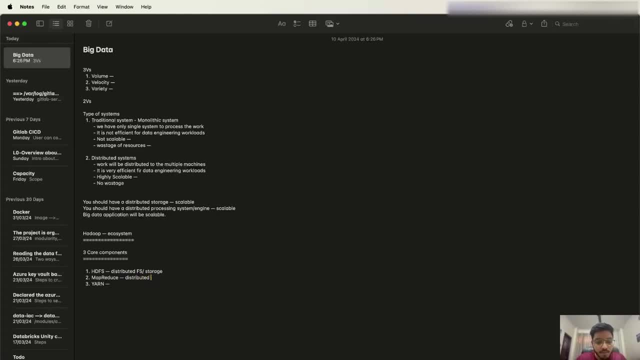 cover, but for now just understand: this is, is is distributed processing engine. processing engine. processing engine: okay, the yarn, okay, the yarn. okay, the yarn. and the next thing is the yarn yarn is, and the next thing is the yarn yarn is, and the next thing is the yarn yarn is. nothing but yet another resource. 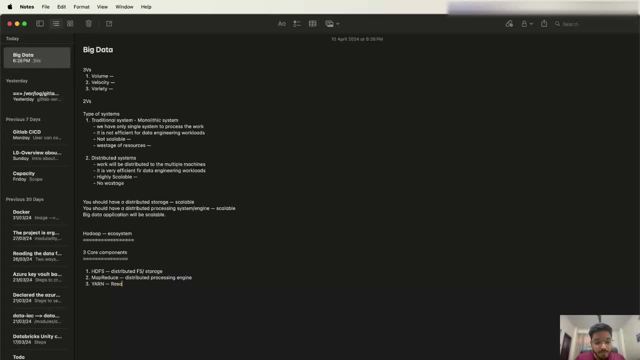 nothing but yet another resource. nothing but yet another resource. negotiator, negotiator, negotiator. so this is a resource manager. so, in the distributed system, what will so in the distributed system? what will so in the distributed system? what will you will be having, you will be having. 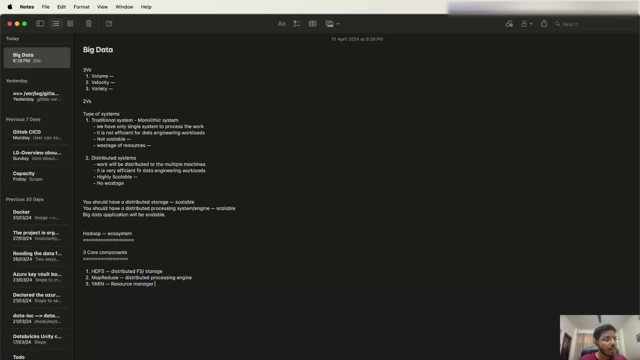 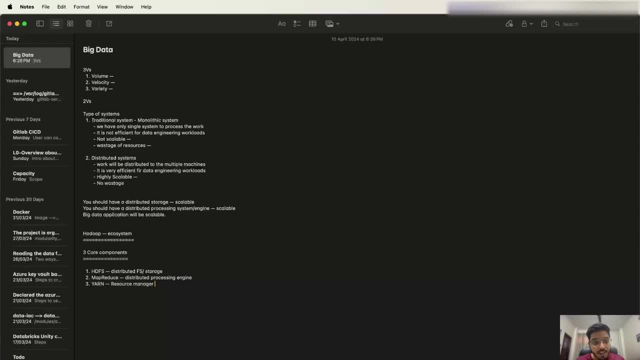 have, let's say, two, two files, let's say 100 gb file, 1 200 gb file. so you will be 100 gb file, 1 200 gb file. so you will be 100 gb file, 1 200 gb file. so you will be creating, let's say, two jobs to process. 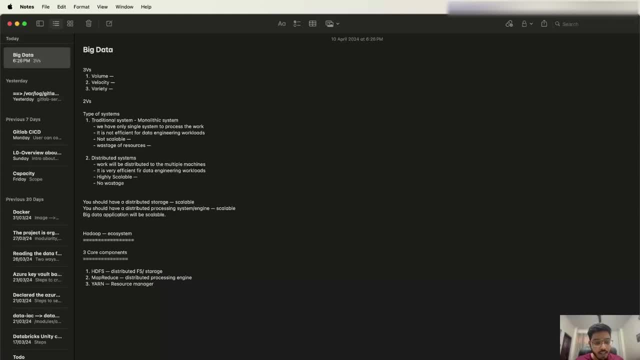 creating. let's say two jobs to process creating. let's say two jobs to process: individual file: okay, two separate jobs, individual file: okay, two separate jobs, individual file- okay, two separate jobs. but the requirement of the machines, but the requirement of the machines, but the requirement of the machines, the number of machines will be different. 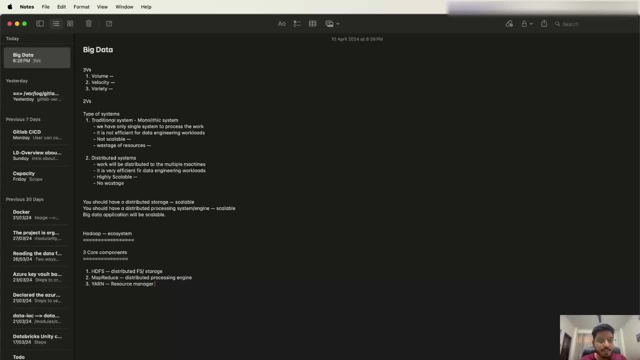 the number of machines will be different. the number of machines will be different- 400 gb file- and will be different for 400 gb file and will be different for 400 gb file and will be different for 200 gb files. let's suppose you need five. 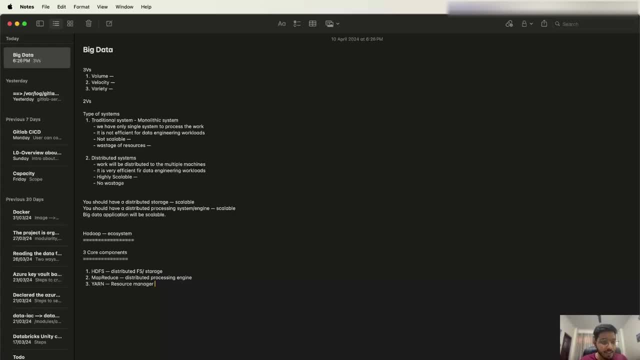 200 gb files. let's suppose you need five 200 gb files. let's suppose you need five machines to process 100 gb file and you machines to process 100 gb file and you machines to process 100 gb file and you need 10 gb. sorry, 10 machines to process. 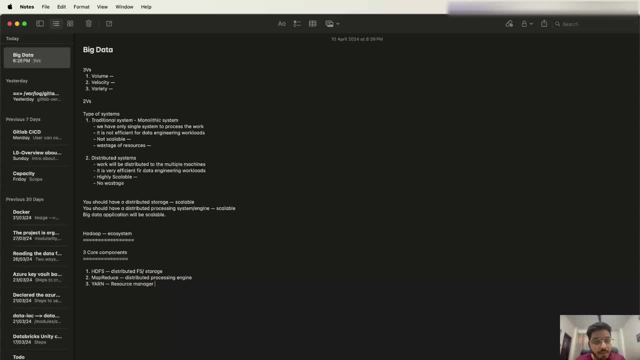 need 10 gb- sorry, 10 machines- to process. need 10 gb- sorry, 10 machines- to process 200 gb file. so you need some program 200 gb file. so you need some program 200 gb file. so you need some program that will basically allocate the. 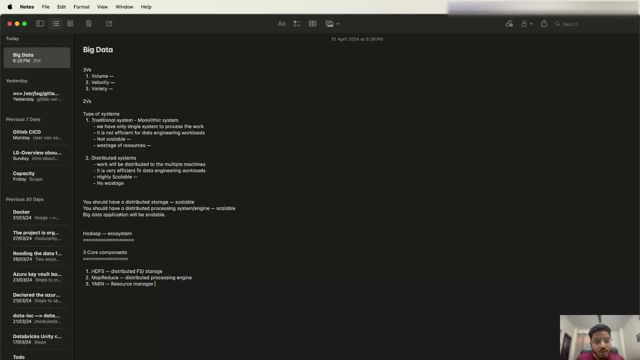 that will basically allocate the. that will basically allocate the resources. manage the resources for these resources, manage the resources for these resources, manage the resources for these different jobs, different jobs, different jobs. so this is the yarn that will take care. so this is the yarn that will take care. 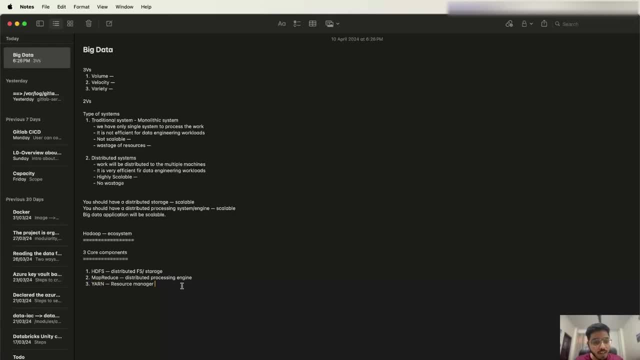 so this is the yarn. that will take care of it. it will see. okay for the job one of it. it will see okay for the job one of it. it will see okay for the job one. job number one is uh to process 100 gb. job number one is uh to process 100 gb. 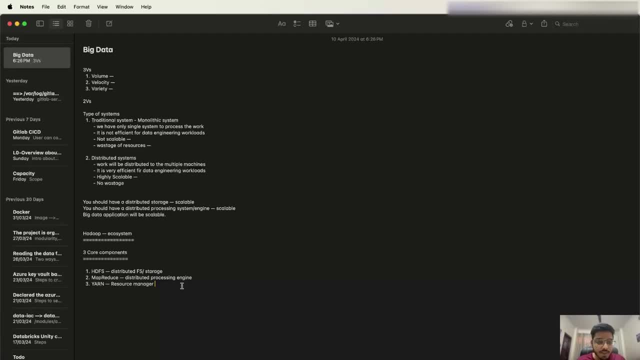 job number one is, uh, to process 100 gb files, so they, so we, we will need let's files, so they, so we, we will need let's files, so they, so we, we will need, let's say five machines, so it will allocate. say five machines, so it will allocate. 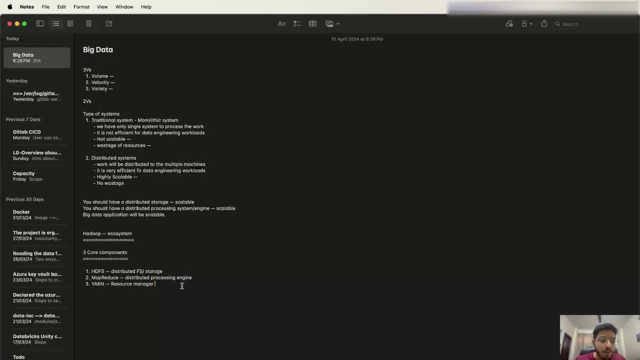 say five machines. so it will allocate the five machines in the distributed, the five machines in the distributed, the five machines in the distributed system, and it will coordinate further system and it will coordinate further system and it will coordinate further, coordinate with those machines like it, coordinate with those machines like it. 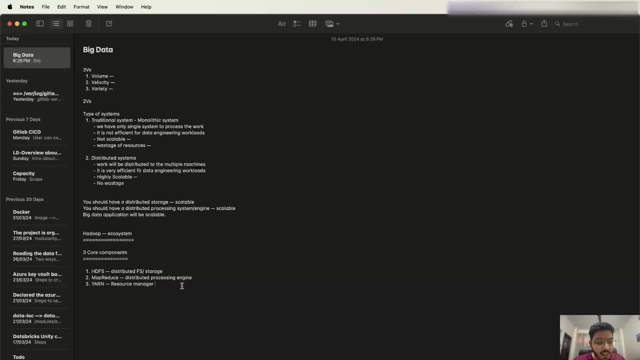 coordinate with those machines. like it will check for the status. what is? will check for the status. what is? will check for the status. what is happening, what is the status of the happening? what is the status of the happening? what is the status of the task? what is the status of the job? 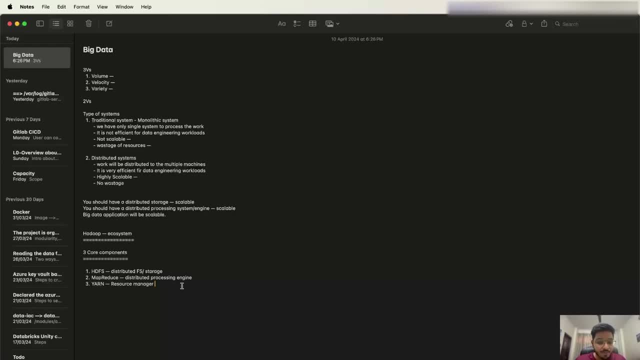 task. what is the status of the job task? what is the status of the job and when the comp, when the job will be and when the comp, when the job will be and when the comp when the job will be completed, it completed, it completed, it, the. the status will be returned like. 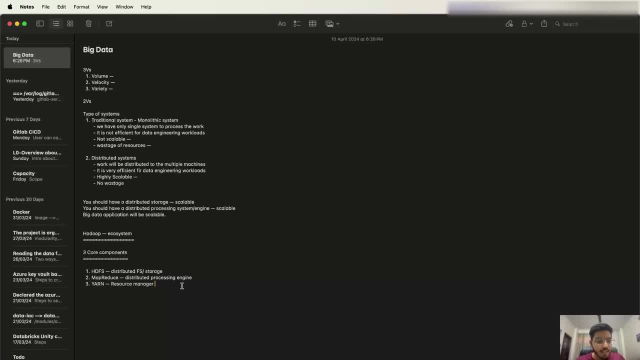 the. the status will be returned like. the. the status will be returned like: send back to the resource manager and send back to the resource manager and send back to the resource manager and further. it will take care of it like. further. it will take care of it like: 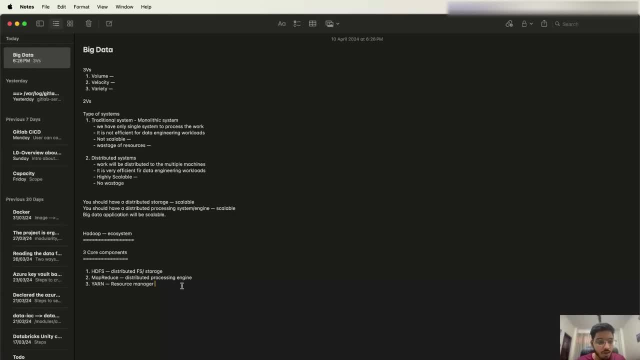 further, it will take care of it like: so this is how the whole whole, so this is how the whole whole, so this is how the whole whole coordination is working with the help of coordination is working with the help of coordination is working with the help of different tools. 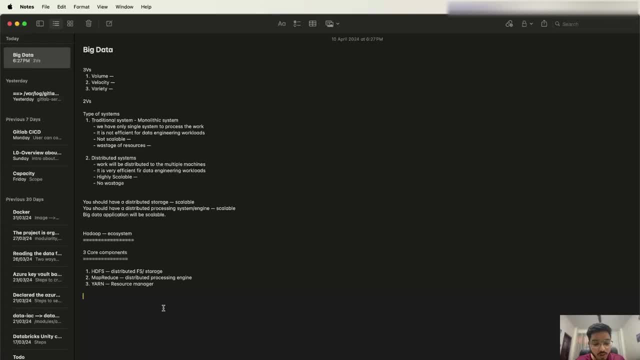 different tools, different tools. so, for example, if you have a machine. so, for example, if you have a machine. so, for example, if you have a machine, let's say you, you are creating a data. let's say you, you are creating a data. let's say you, you are creating a data pipeline or a data application. so there, 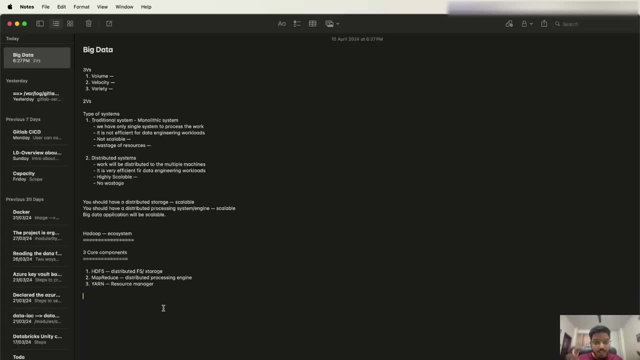 pipeline or a data application. so there pipeline or a data application. so there will be some resources. there will be will be some resources. there will be, will be some resources. there will be some processing engine and storage. let's some processing engine and storage. let's some processing engine and storage. let's suppose, so suppose, you have the data. 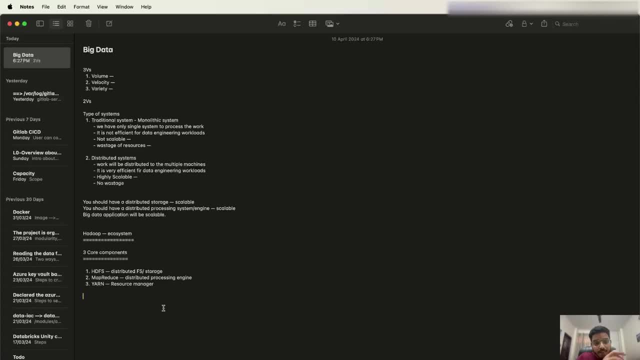 suppose so, suppose you have the data, suppose so, suppose you have the data stored on different data sources, so you stored on different data sources, so you stored on different data sources. so you need some tool that will need some tool that will need some tool that will, that will basically extract the data from. 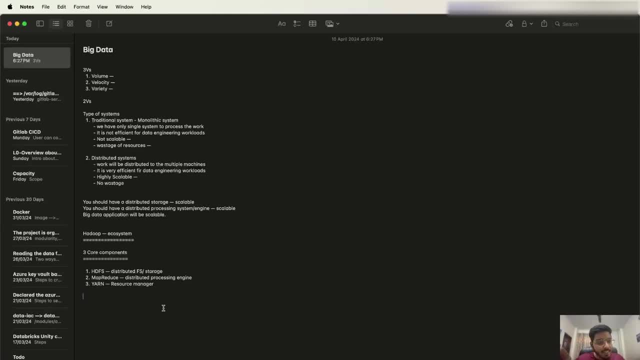 that will basically extract the data from. that will basically extract the data from those resources data sources and put those resources data sources and put those resources data sources and put that data inside the sdfs so that it can, that data inside the sdfs so that it can. 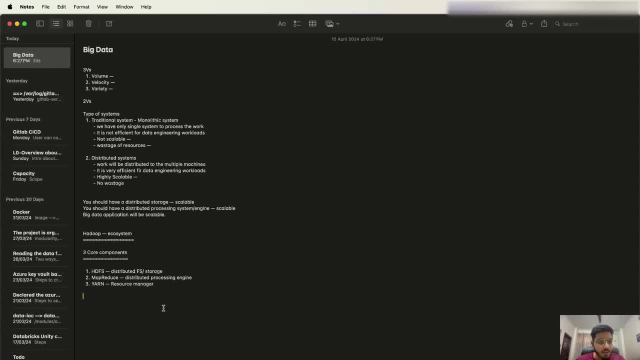 that data inside the sdfs, so that it can be further processed by the map reduce, be further processed by the map reduce, be further processed by the map reduce. okay, so this, uh, there is a tool that is okay. so this, uh, there is a tool that is. 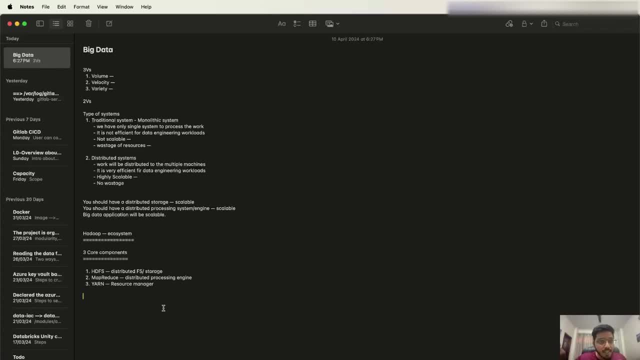 okay, so this, uh, there is a tool that is required that will extract the data from required, that will extract the data from required, that will extract the data from the sources and put putting that data the sources and put putting that data the sources and put putting that data inside the sdfs. so, for this use case, we 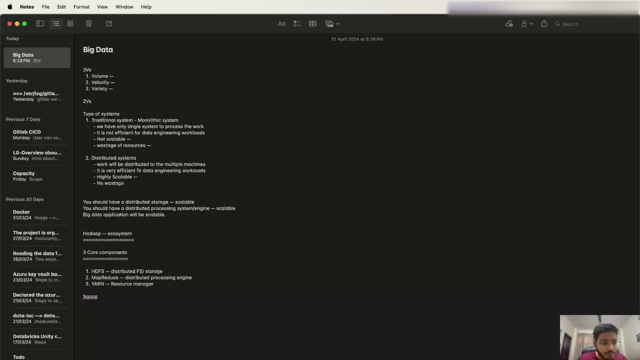 inside the sdfs. so for this use case, we inside the sdfs. so for this use case, we have scoop, have scoop, have scoop, we have scoop. so scoop is basically: we have scoop, so scoop is basically we have scoop, so scoop is basically ingestion tool, ingestion tool. 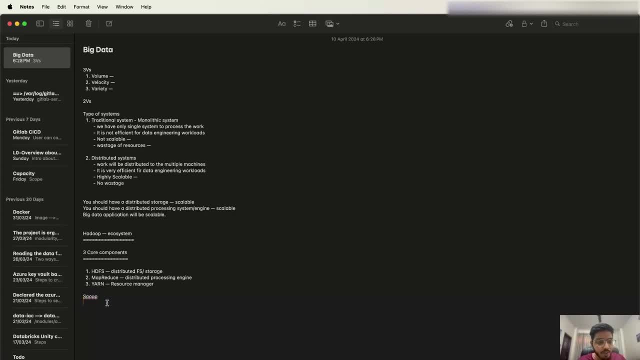 ingestion tool. uh, we will uh see uh. i'm just giving an. uh, we will uh see uh. i'm just giving an. uh, we will uh see uh. i'm just giving an overview of the tools. the name of the overview of the tools. the name of the. 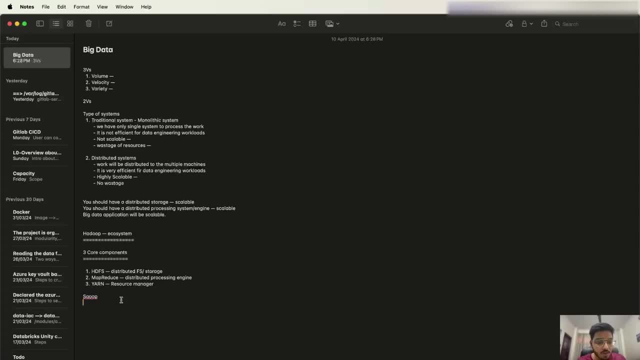 overview of the tools, the name of the tools: uh, what are the important tools tools? uh, what are the important tools tools? uh, what are the important tools? i'll cover, uh those tools only. what will i'll cover, uh those tools only. what will i'll cover? uh those tools only? what will be required in your interview and in the 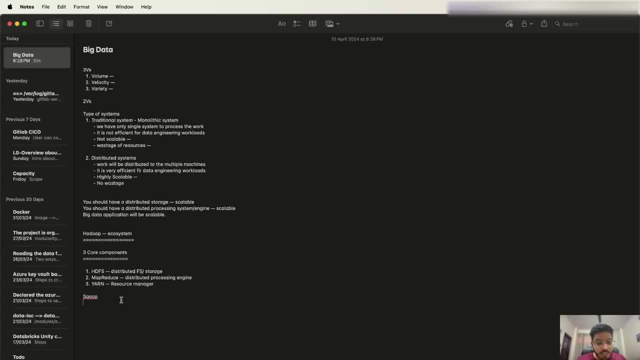 be required in your interview and in the be required in your interview and in the day-to-day jobs, basically like: uh, so day-to-day jobs. basically like: uh, so day-to-day jobs. basically like: uh, so scoop is nothing but ingestion tool. then scoop is nothing but ingestion tool. then. 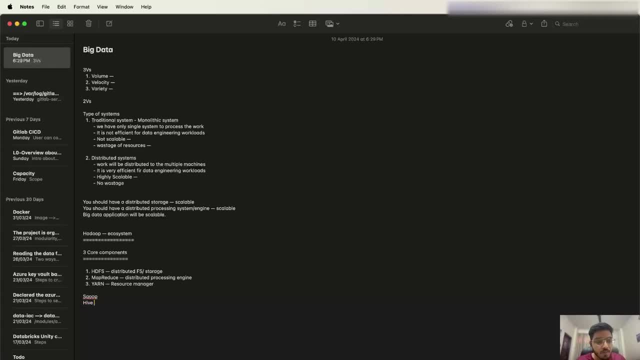 scoop is nothing but ingestion tool. then we have hive, we have hive, we have hive. hive is uh. so once you have processed your hive is uh. so once you have processed your hive is uh. so once you have processed your data, that is like present uh in some. 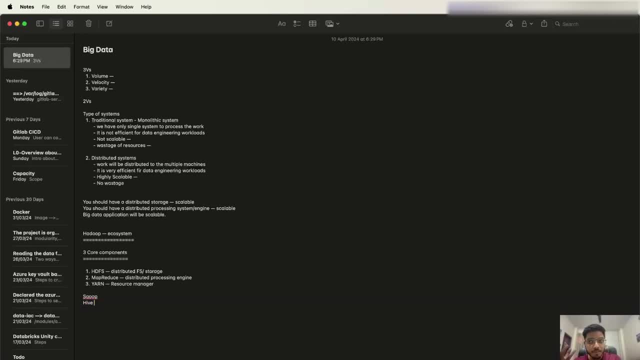 data that is like present, uh, in some data that is like present, uh, in some storage. so you need some engine, some storage. so you need some engine, some storage. so you need some engine, some, uh, basically, uh, basically, uh, basically data warehousing tool so that you can. 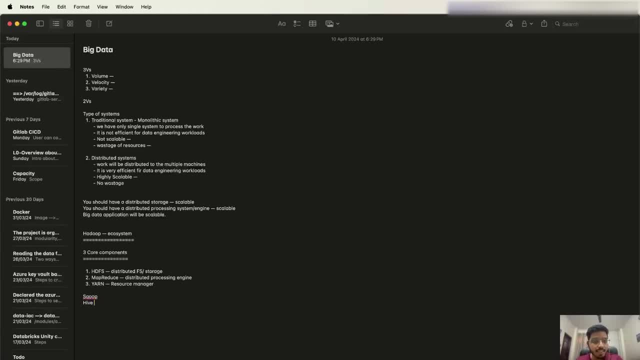 data warehousing tool so that you can. data warehousing tool so that you can write some queries, analyze your data. write some queries, analyze your data, write some queries, analyze your data- okay, and run some aggregation on your on, okay, and run some aggregation on your on, okay, and run some aggregation on your on top of your data. so you need some tool. 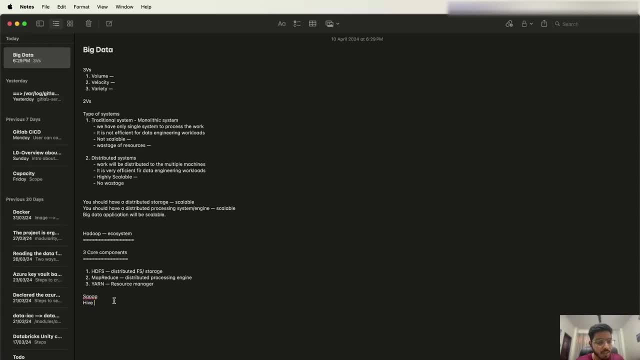 top of your data, so you need some tool. top of your data, so you need some tool. so for that people have created hive hive. so for that people have created hive hive. so for that people have created hive. hive is again open source, is again open source, is again open source. so hive is basically uh. 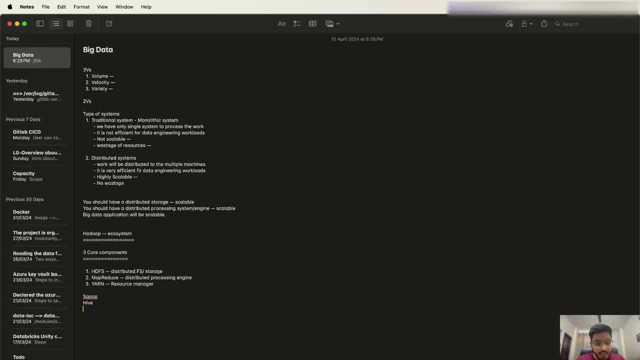 so hive is basically uh, so hive is basically uh, your data warehousing tool, your data warehousing tool, your data warehousing tool. then we have something called uh, then we have something called uh, then we have something called uh, pig, we have pig, we have pig, we have, we have. 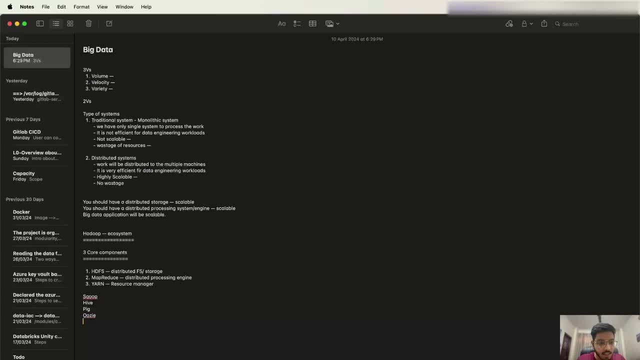 oozy, oozy, oozy. i'm not sure if the spelling is correct. i'm not sure if the spelling is correct. i'm not sure if the spelling is correct. you can check. so there are like similar- you can check. so there are like similar, you can check. so there are like similar multiple tools that are helping us for a. 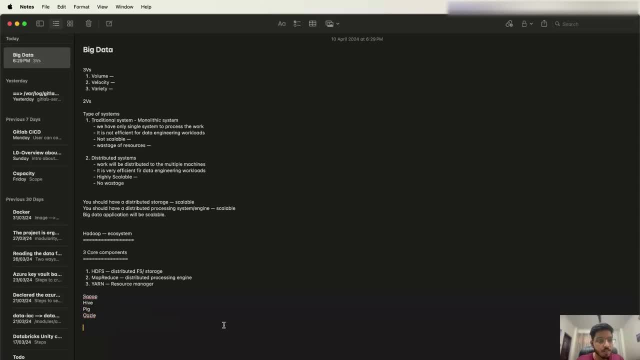 multiple tools that are helping us for a multiple tools that are helping us for a different use cases. okay, so this is different use cases. okay, so this is different use cases. okay, so this is about the about the, about the tools. we have tools we have, tools we have. so there are like a lot of, lot of tools. 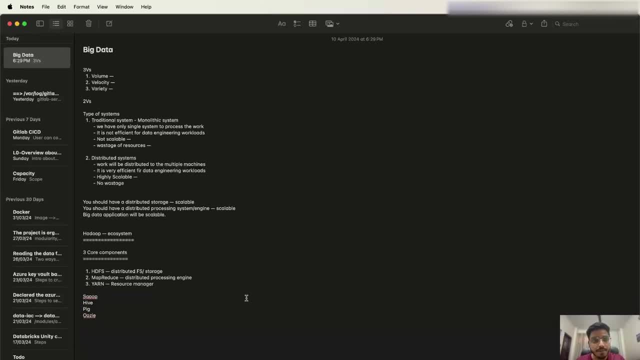 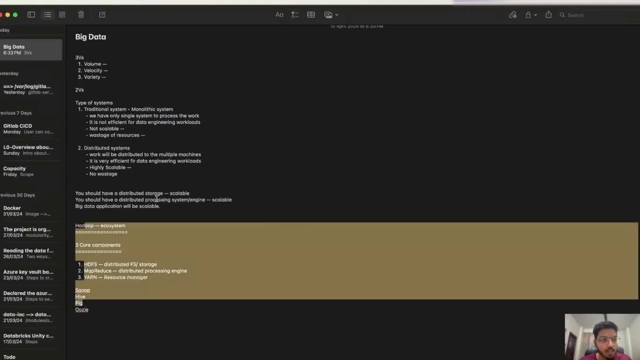 so there are like a lot of lot of tools. so there are like a lot of lot of tools available, but we will be covering what available. but we will be covering what available, but we will be covering what is required. is required, is required. okay, so we have covered hadoop and 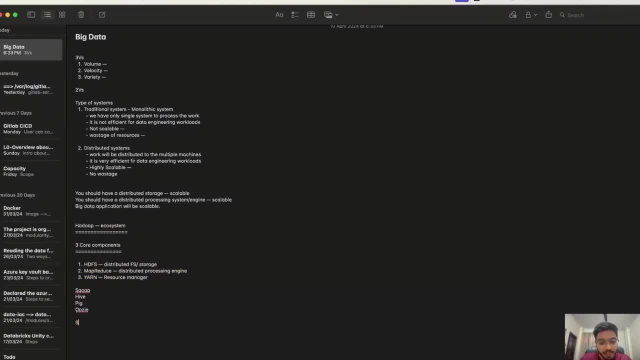 so we have covered hadoop, and so we have covered hadoop, and so there is a one more: uh, basically the. so there is a one more, uh, basically the. so there is a one more, uh, basically the main, main, main. so there is a spark. this is another. 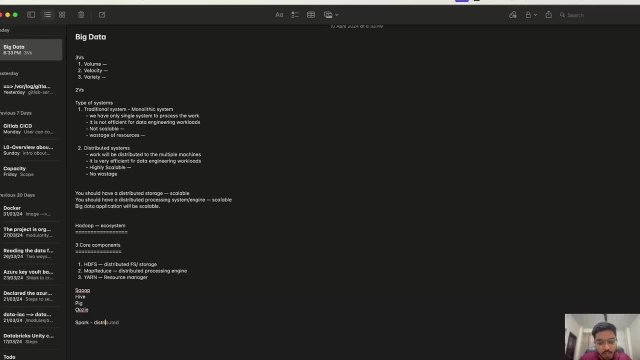 so there is a spark. this is another. so there is a spark. this is another processing engine: distributed processing processing engine. distributed processing processing engine. distributed processing, basically distributed processing, basically distributed processing, basically distributed processing engine, engine, engine, so so, so, like this is the processing engine that is. 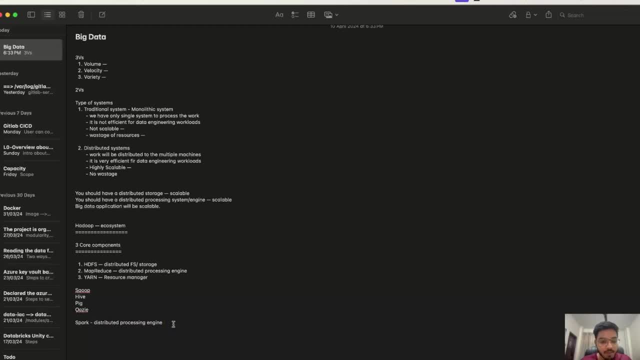 like: this is the processing engine that is like: this is the processing engine that is currently like, currently like, currently like, used by most of the companies. i would say used by most of the companies. i would say used by most of the companies, i would say the almost of all the companies. 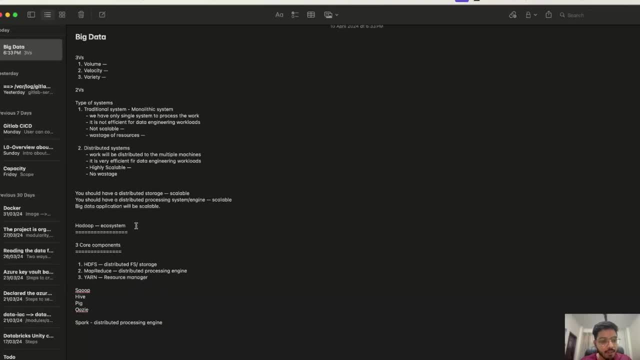 the almost of all the companies, the almost of all the companies, and, and, and. so there are some challenges that we so, there are some challenges that we so there are some challenges that we were facing in hadoop, were facing in hadoop, were facing in hadoop, and, uh, that are, you can say, resolved by. 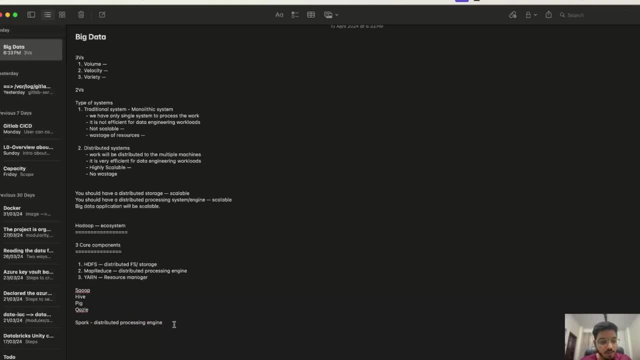 and uh that are, you can say resolved by, and uh that are, you can say resolved by spark and spark and spark and so so. so what are the differences? uh? so, what are the differences? uh? so what are the differences, uh? so, basically, if you see hadoop, uh, hadoop. 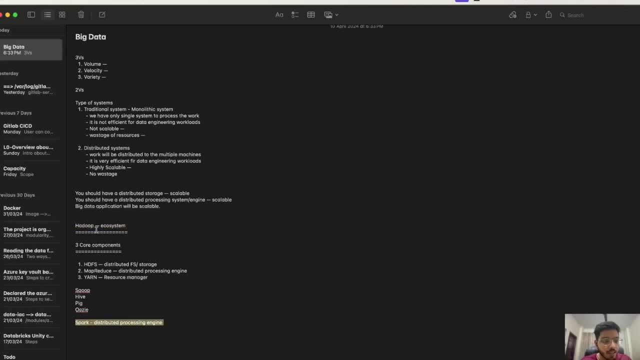 basically, if you see hadoop, uh hadoop. basically, if you see hadoop, uh hadoop, you cannot compare hadoop with spark, you cannot compare hadoop with spark, you cannot compare hadoop with spark. hadoop, as i mentioned, hadoop is a hadoop. as i mentioned, hadoop is a. 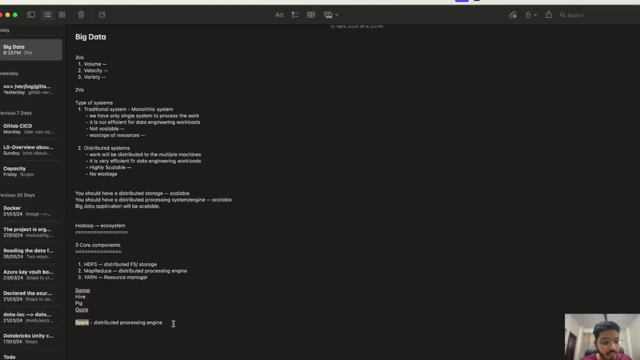 hadoop. as i mentioned, hadoop is a ecosystem, it is not a tool ecosystem. it is not a tool ecosystem. it is not a tool. but spark, i would say, is directly a, but spark, i would say is directly a, but spark, i would say, is directly a processing engine. 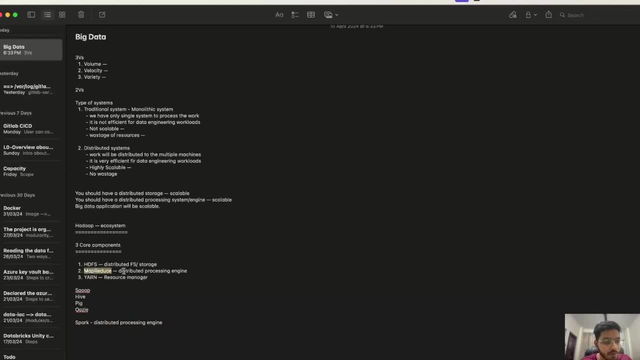 processing engine, processing engine. spark is compared, can be compared with spark is compared, can be compared with spark is compared, can be compared with map reduce, because map reduce is a map reduce, because map reduce is a map reduce, because map reduce is a processing engine, processing engine, processing engine. you cannot say spark versus hadoop you. 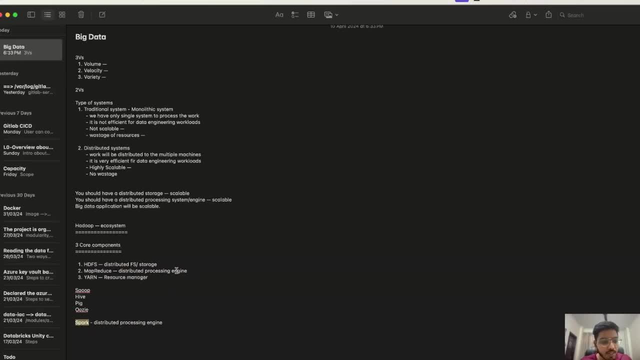 you cannot say spark versus hadoop you. you cannot say spark versus hadoop. you can say spark versus map. reduce. so map can say spark versus map. reduce. so map can say spark versus map. reduce. so map reduce in the processing engine. spark is reduce in the processing engine. spark is. 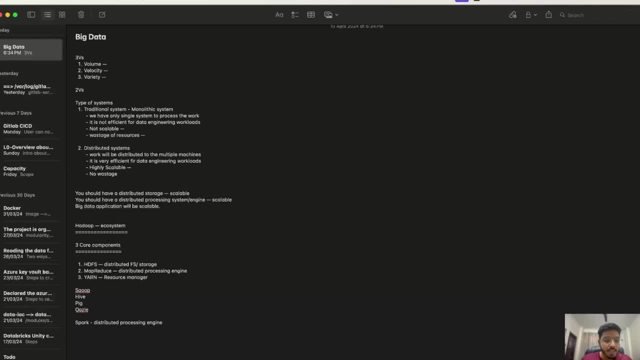 reduce in the processing engine. spark is a processing engine distributed, a processing engine distributed, a processing engine distributed. processing engine, processing engine, processing engine. so there are some challenges that we were, so there are some challenges that we were, so there are some challenges that we were facing in the 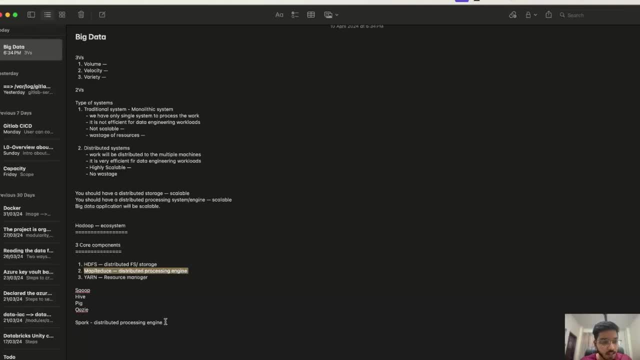 facing in the facing in the. you know uh map reduce and you know uh map reduce and you know uh map reduce, and and those challenges are basically solved, and those challenges are basically solved, and those challenges are basically solved by the, by the, by the spark, uh okay. 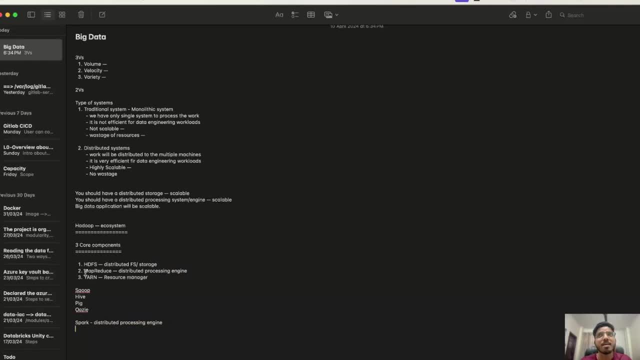 spark, uh okay, spark, uh okay. so so basically uh at high level, uh i. so so basically uh at high level, uh i. so so basically uh at high level. uh, i would say, would say would say: the map reduce is a, the map reduce is a, the map reduce is a disk based. 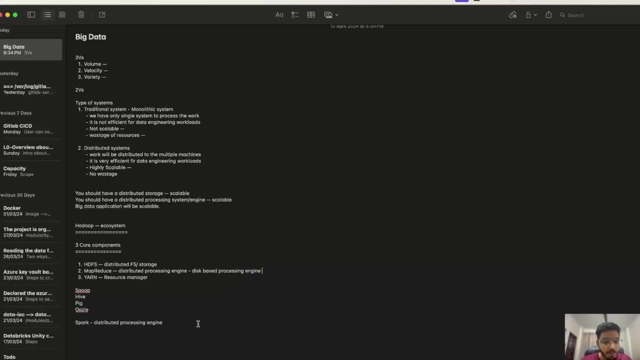 disk based, disk based processing. processing. processing engine: okay. engine: okay. engine, okay, but but. but the spark is in memory. the spark is in memory, the spark is in memory. processing engine: processing engine: okay, processing engine, okay, so, so. so it is where the, it is where the, it is where the big difference basically come. 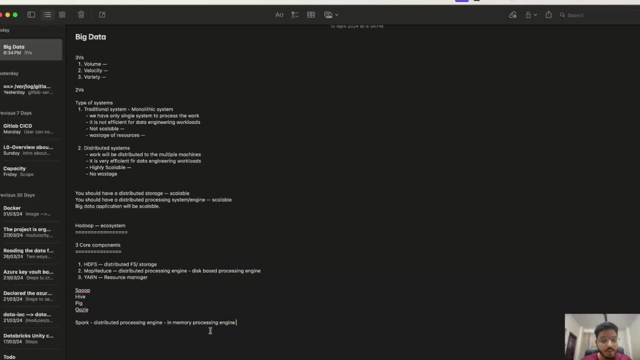 big difference basically come. big difference basically come when we compare to both of these, when we compare to both of these, when we compare to both of these. so we will be covering everything. so we will be covering everything, so we will be covering everything in detail, but for now, 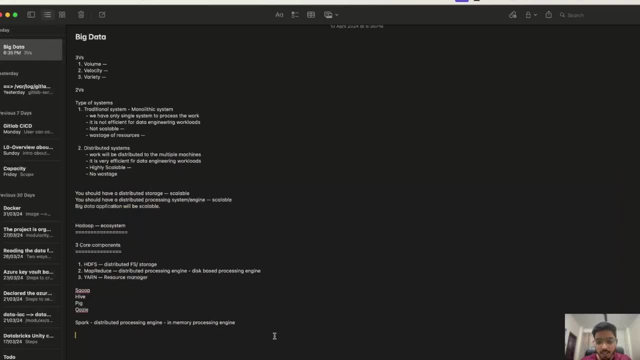 in detail, but for now, in detail, but for now, it was just a high level overview. it was just a high level overview, it was just a high level overview and let's and let's and let's see, see, see, let's meet in the next, next lecture. okay, let's meet in the next next lecture. okay,